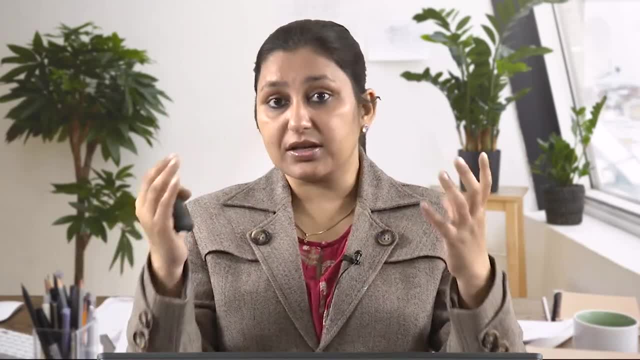 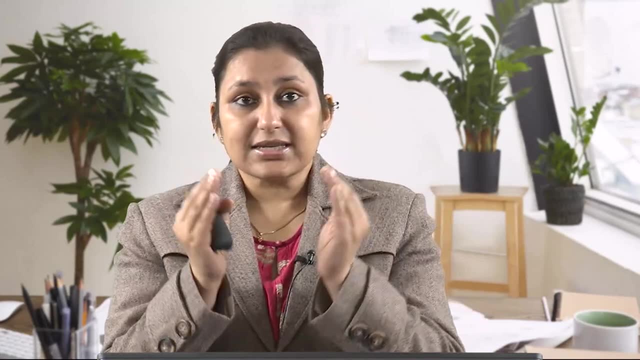 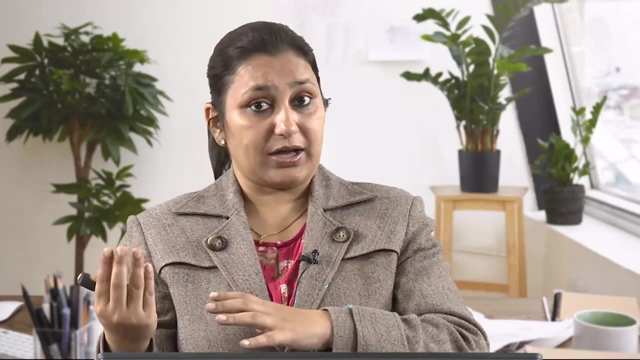 Okay, I want a toy which is a spherical toy. So there is a design which is conceived in the minds of the designer Once it has been conceived. after that it is further designed and analyzed that how will it be manufactured. So the third stage goes on to manufacturing. 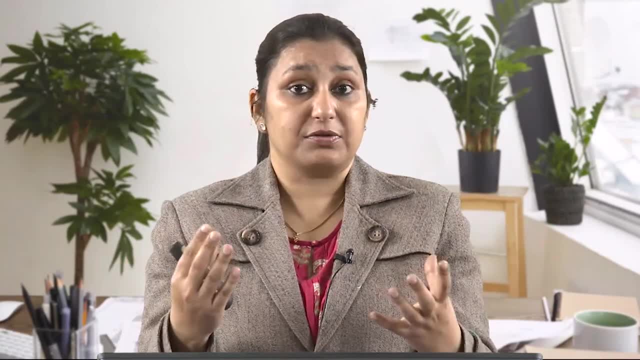 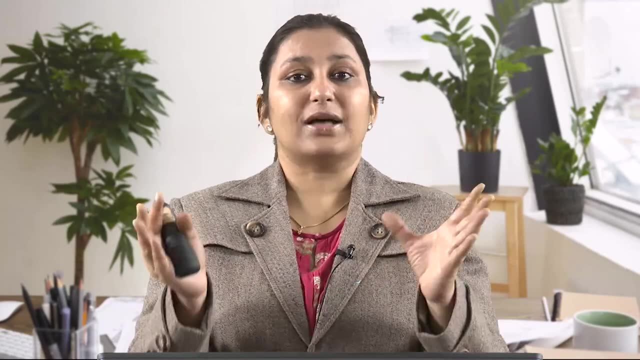 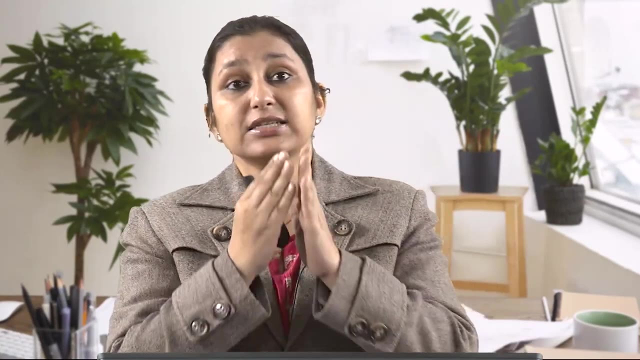 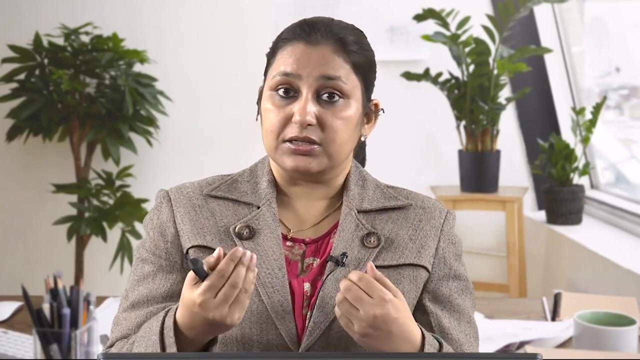 And then, once it is manufactured, it is verified whether it will work the way it was intended to be designed or not. And once it has been verified, it is out as a product used by people and, finally, we dispose it off. At each one of these stages, we require to communicate our ideas. 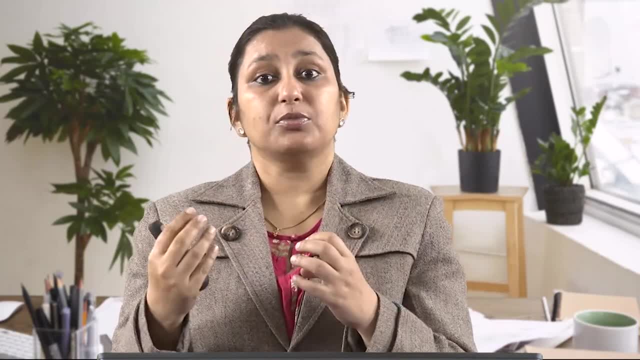 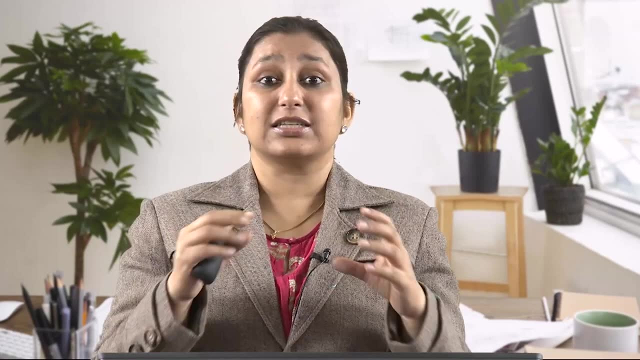 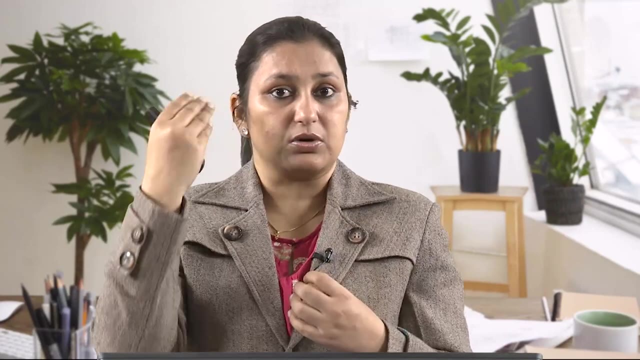 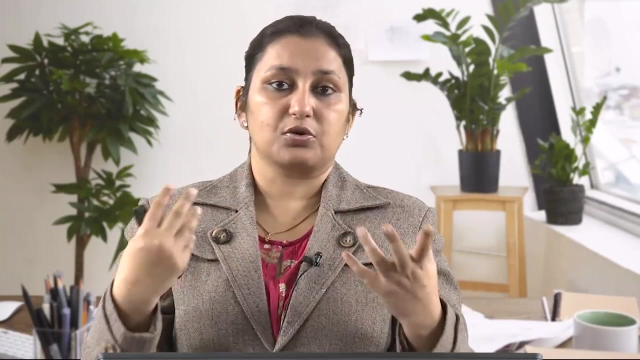 so at the conception stage, we require to communicate what is conceived as an idea. At the design stage and the analysis, we need to communicate how exactly, what are the dimensions, how exactly it is being designed, So what our initial idea was, how will it be designed and analyzed And then to manufacture, if we have to cast a die or whatever. 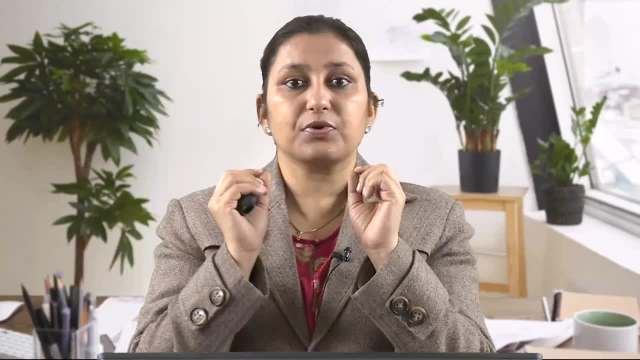 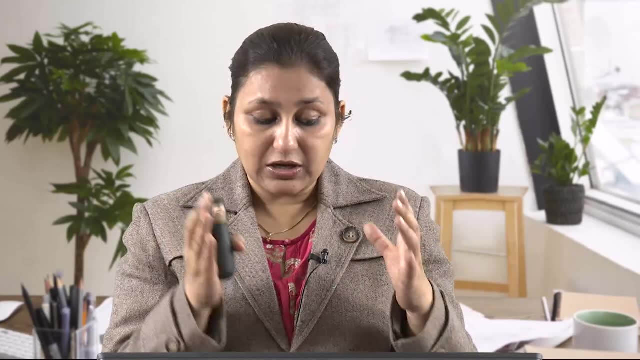 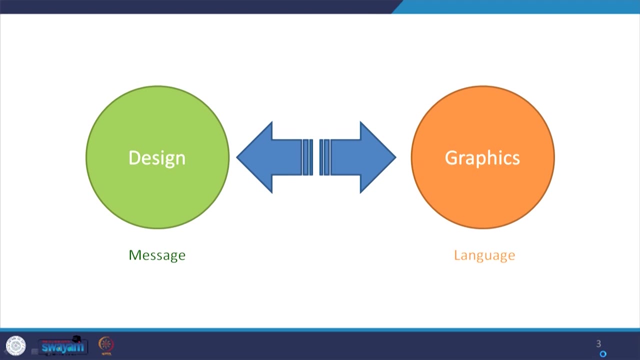 So at each one of these stages, we need to have a precise communication of this idea for the next stage to progress. So if we look at this design, the final design is actually the message. It is only the message and the language in which this message 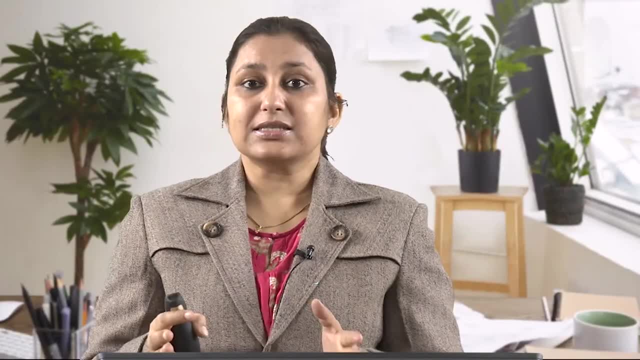 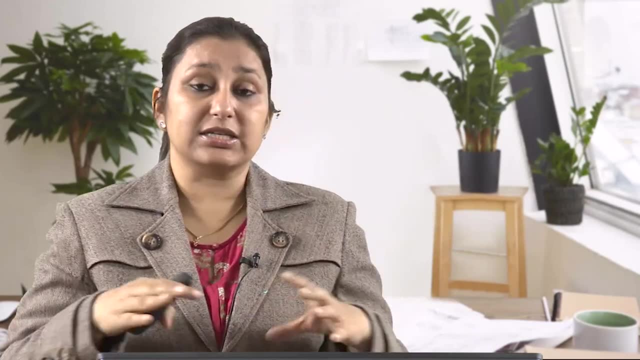 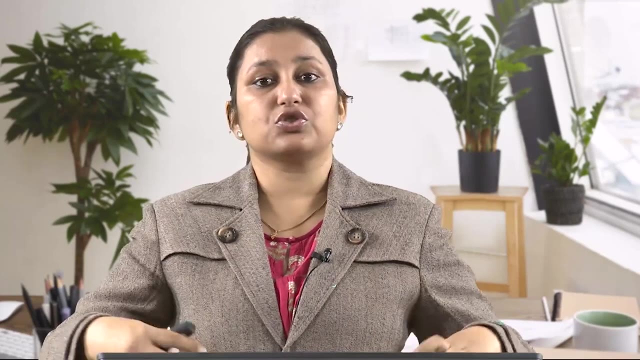 is conveyed is graphics. So basically, graphics is actually a language. So when I am talking to you, when I am communicating all of this, just imagine if there was not the screen, if there was not a graphics which is on the screen in the presentation, and if 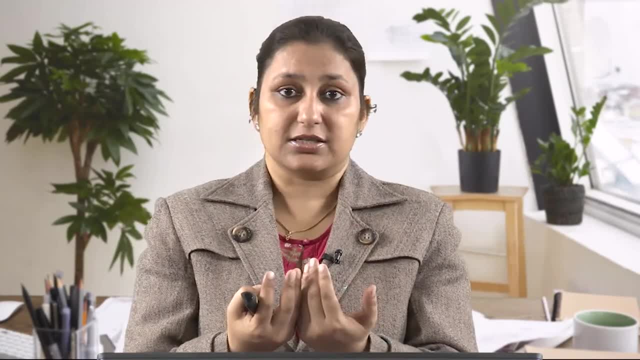 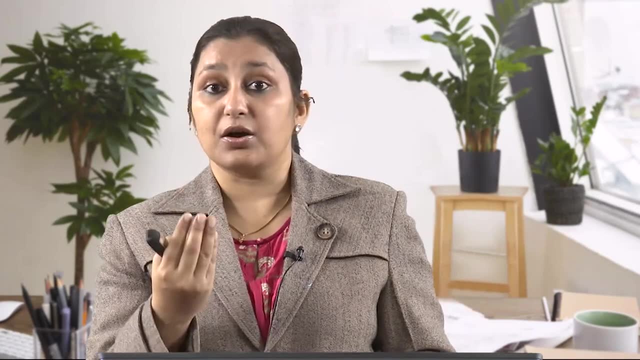 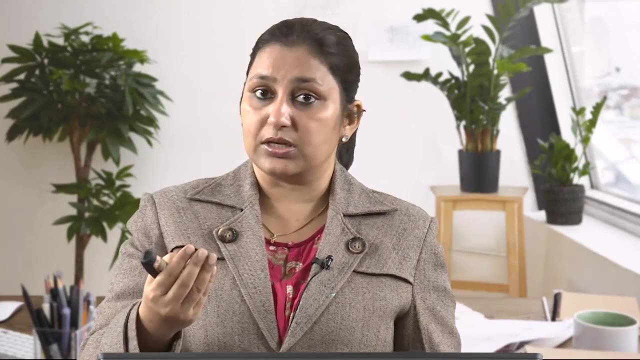 I was only talking through words. I was still communicating. So we are communicating. I am conveying my idea of graphics through a language which is being heard, which is composed of words, sentences, and I am communicating. I could do the same thing, or maybe mix both of these, with the help of this. 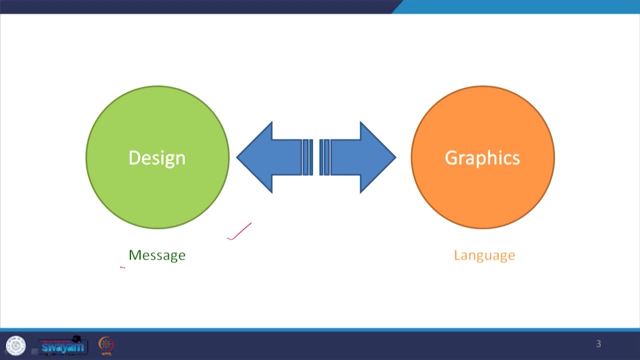 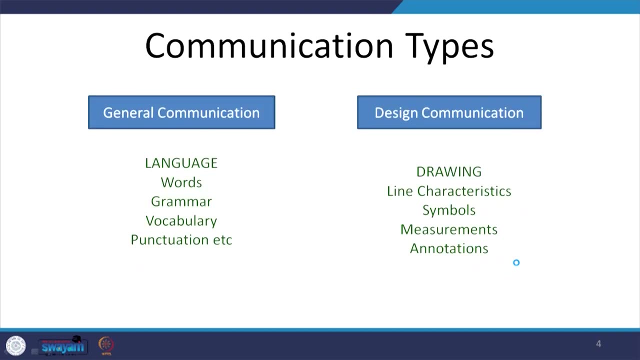 So I have a circle drawn here and I tell you that design is a message and graphics is actually the language to communicate that message. So it is basically language and it is used to communicate. So, if you look at communication types, which is what I have just said, we basically have 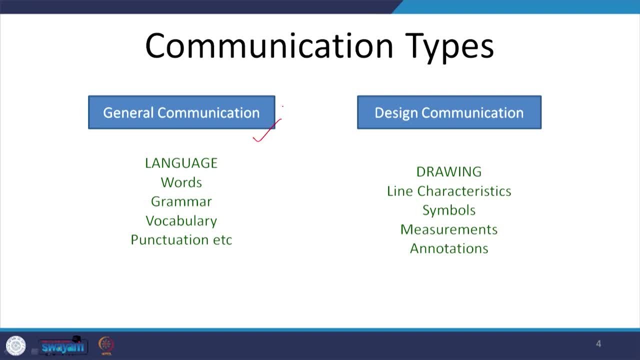 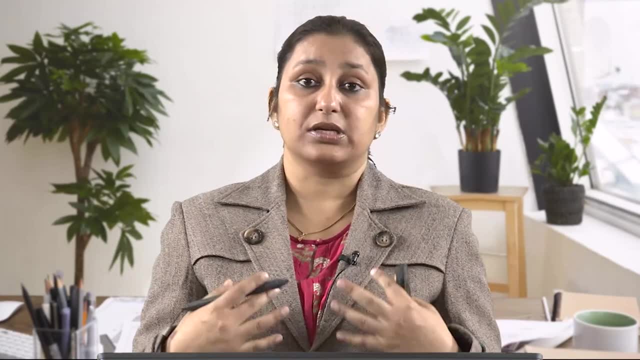 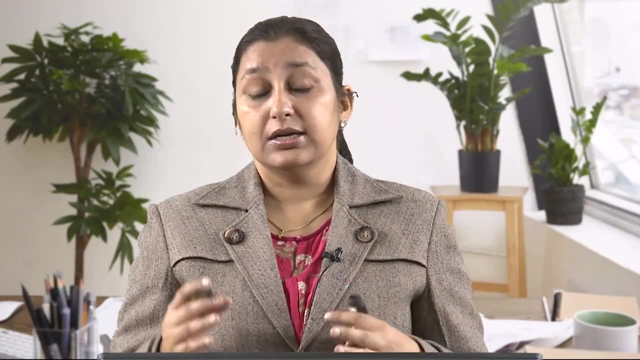 two types of communications. We have a general communication and we have a design communication. If you look at it, If you look at general communication, so all the languages that we read, that we study, for example, Hindi, English, whatever language you might be talking about, it is a way of 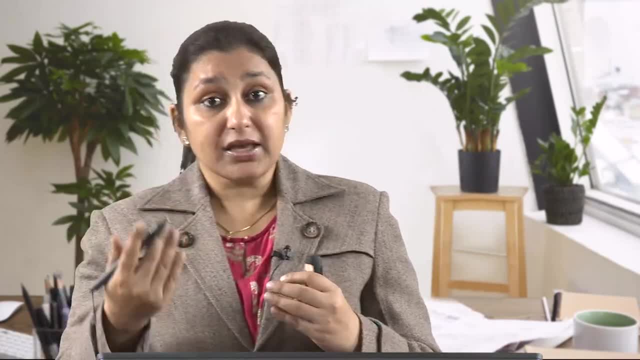 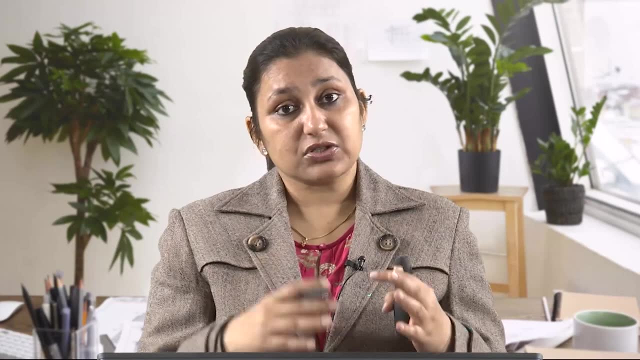 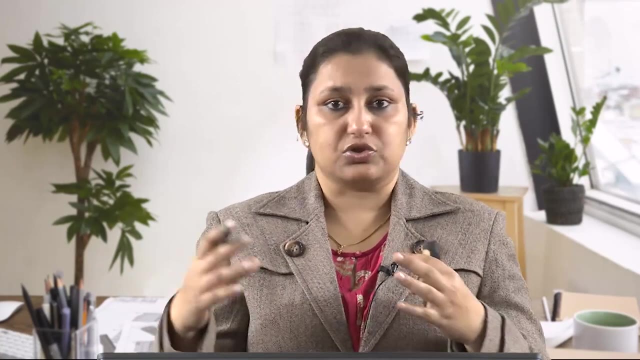 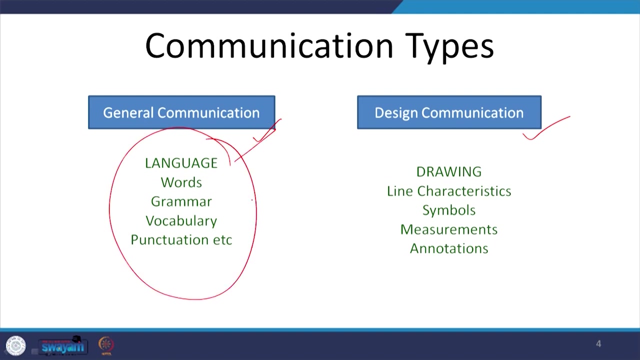 communicating in general. We could speak, we could write through this language. and what this language is comprised of: It has words, it has its own grammar, It has vocabulary, It has punctuation, etc. Exactly all these same components which are part of the general communication. they can. 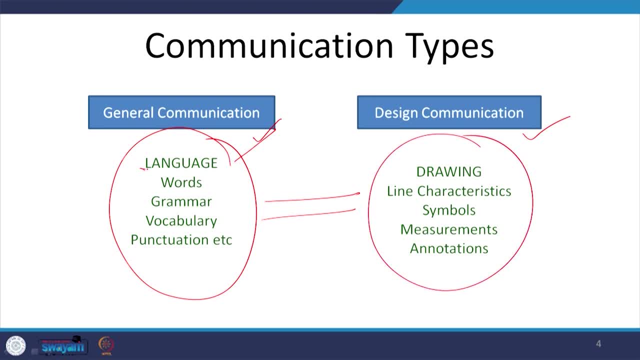 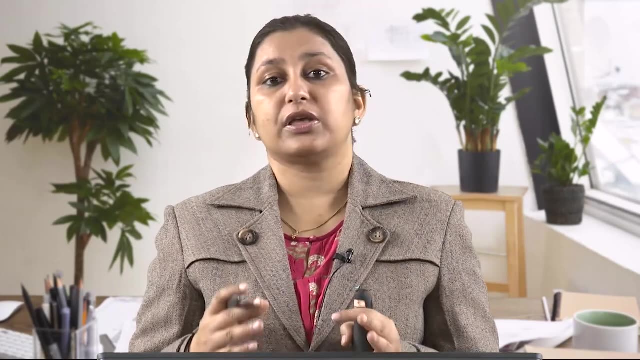 be equated with design communication. So if we talk about language here in general communication, it is the drawing. So what you understand as a language is what you understand through a drawing, and drawing is the language of engineers and architects And, in fact, 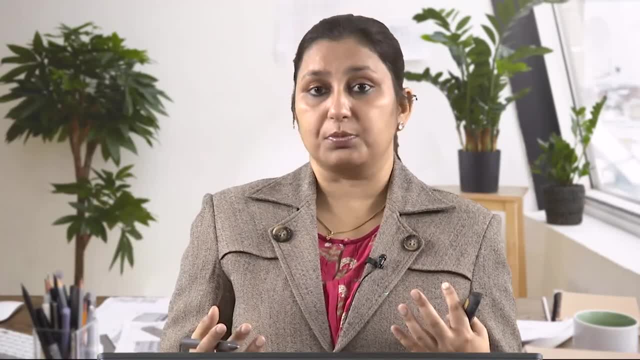 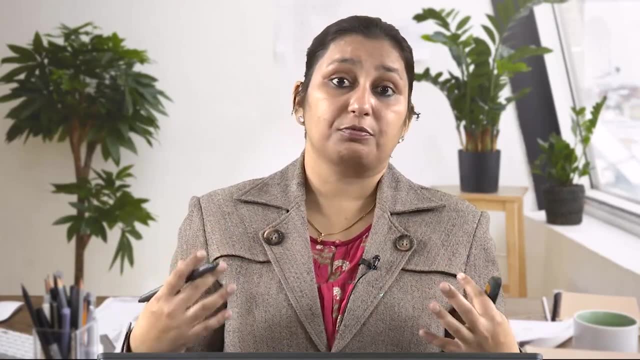 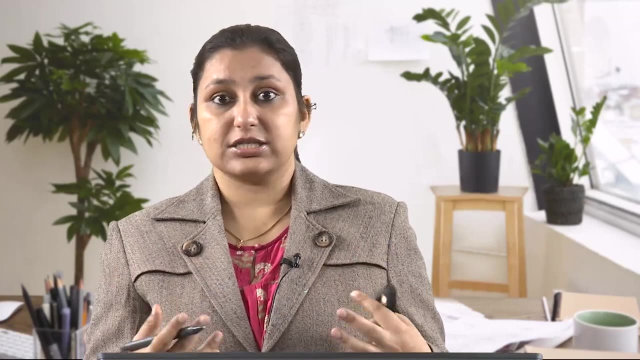 Not really just engineers and architects. primitive people used to communicate through drawings and we have seen that. we have seen those old cave paintings through which they were actually communicating about the lifestyle that they had. So sociologists and historians have been able to deduce a lot of things from the drawings. 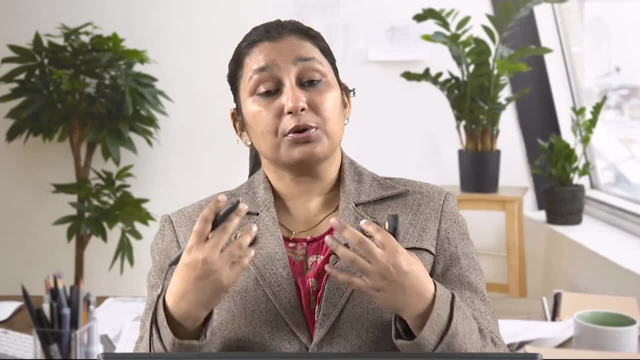 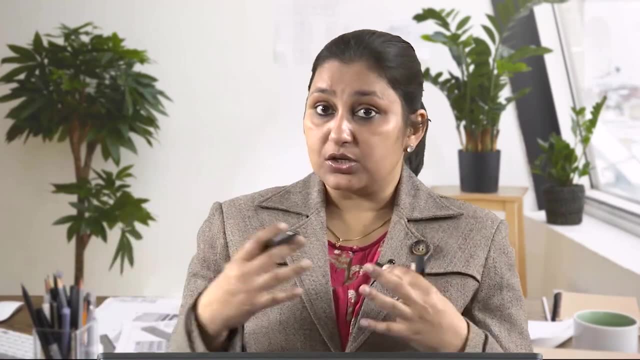 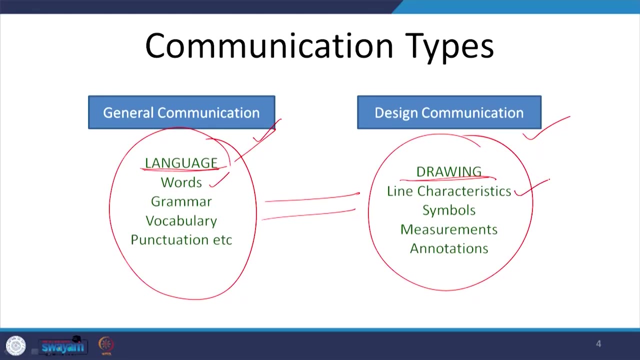 that the prehistoric people, The primitive people in prehistoric times, were able to make- make. So language can be compared with drawing for engineers and architects. Like we have words, we have these different line characteristics. So, for example, we have these different words. 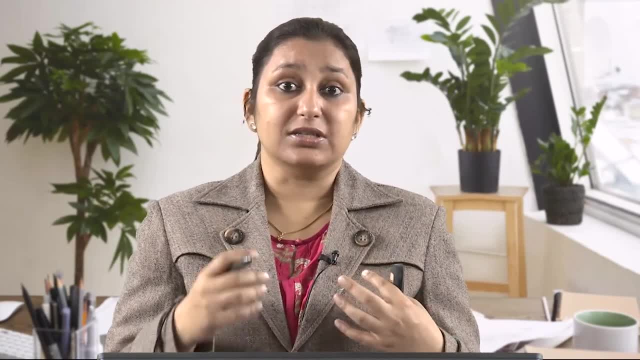 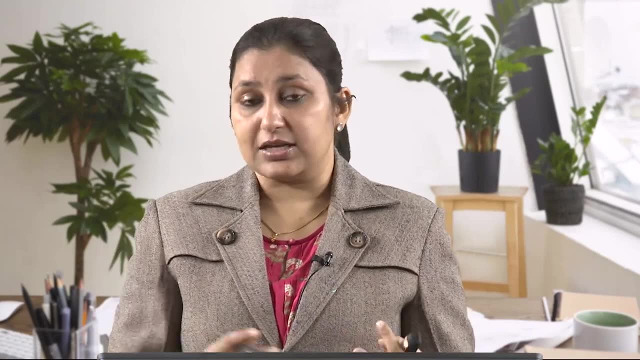 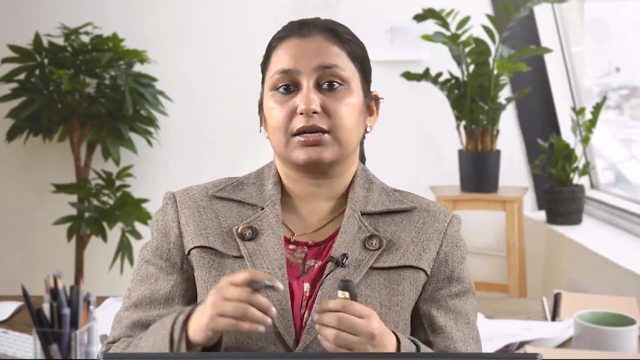 as I am speaking, So I speak, I use these words. speak and draw and communicate, these are all words. Similarly, we have line characteristics. as we go forward in this course, we would see: there is a continuous thick line, there is a continuous thin line, there is a dotted line. 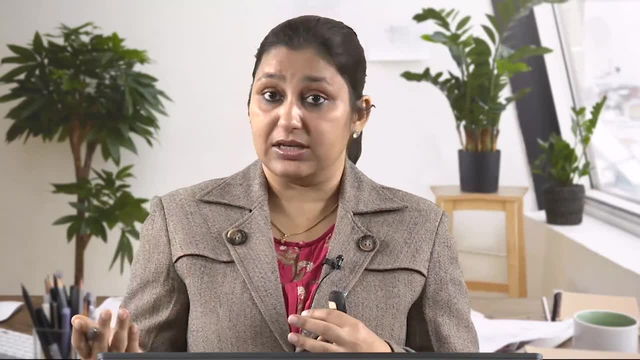 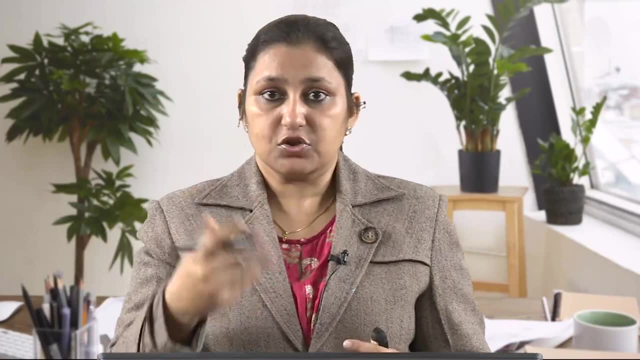 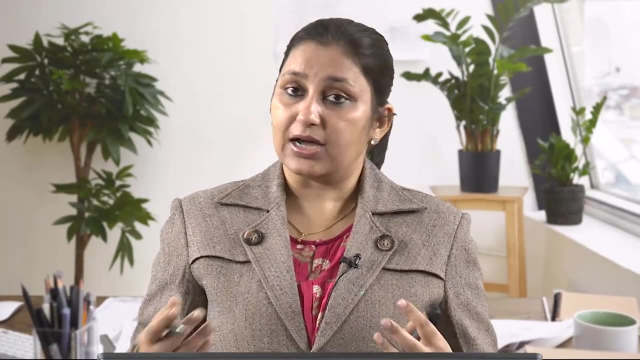 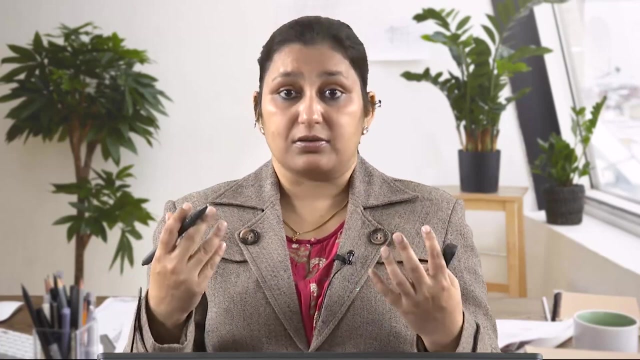 there is a dashed line, and each one of this has a different meaning, just as we have these different words which have different meanings. For example, speak to say continuous line is a solid object, it is a continuous edge being represented. and likewise, just like we have grammar, we have these symbols here. So how do you represent a fan which is going? 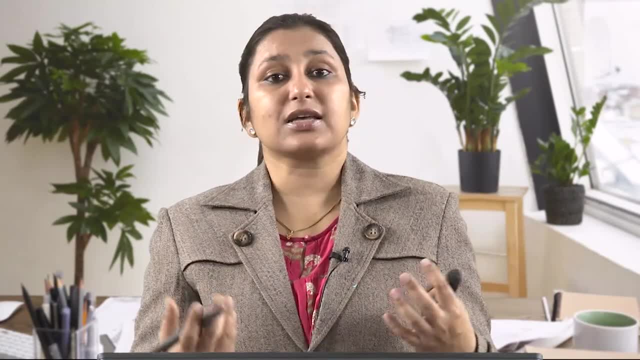 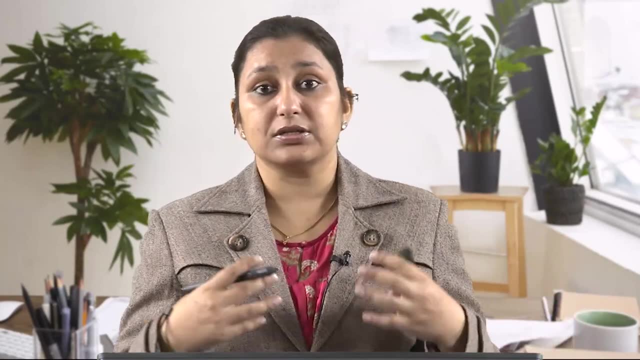 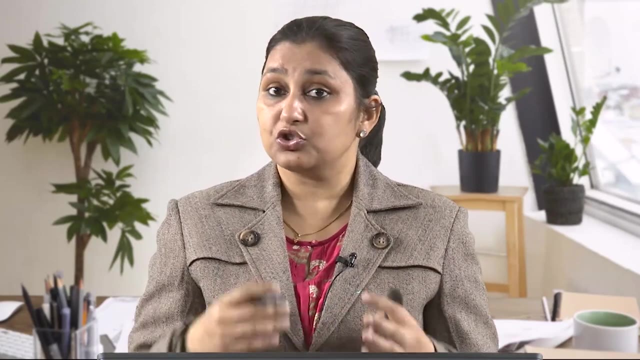 to be placed in a ceiling. there is a symbol for it and it is kind of standard. How do you represent a tap? How do you represent a staircase? How do you represent a cutout in the roof? Each one of these, they have standardized symbols and we use the same symbol. So just 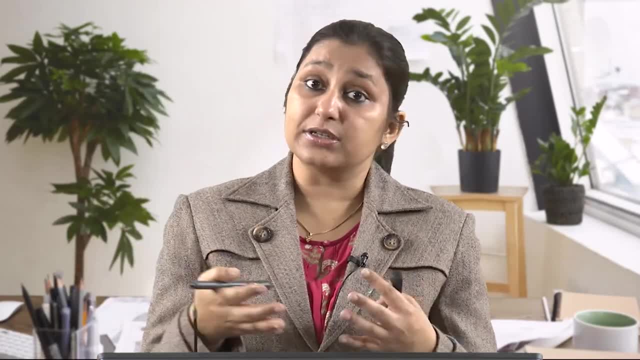 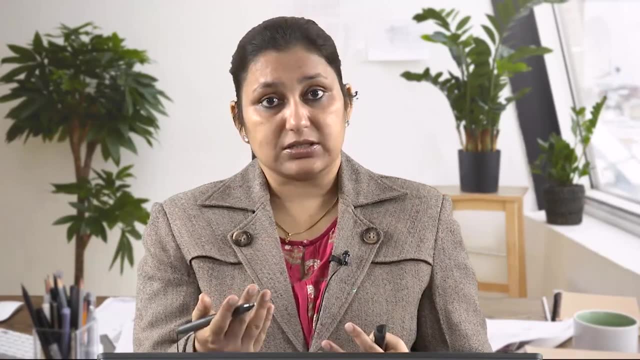 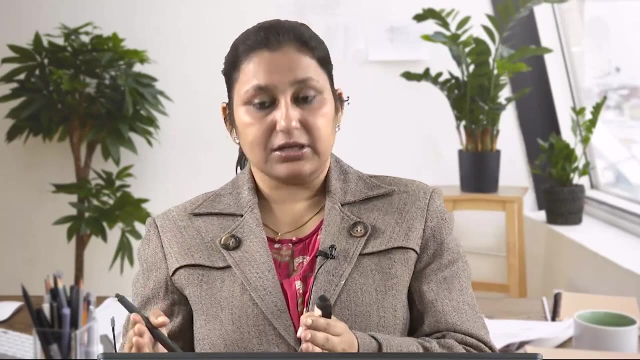 as you understand grammar, how to put these words together. we use symbols, how to put all these different lines together to represent meaning, communicate meaning, Meaningful things, and it is all standard. So grammar is just like grammar is standard. similarly, symbols are standard. Next, we have vocabulary. So we have so many words, so many. 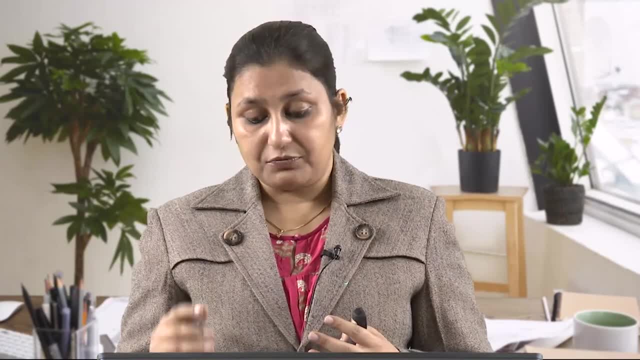 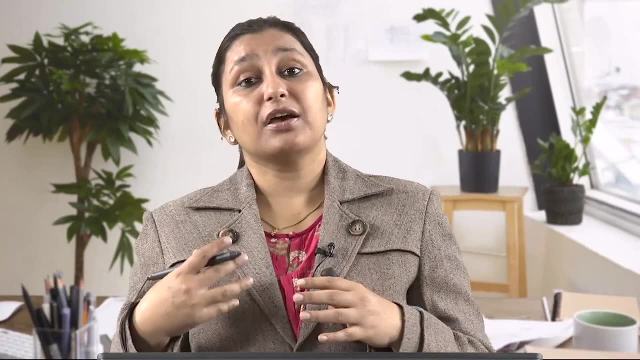 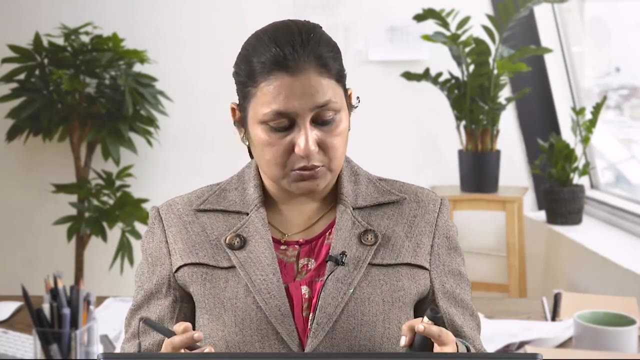 different words for different things. Similarly, we have measurements not exactly equating to vocabulary, but we have measurements to actually communicate the sense of scale: how big or how small is this going to be? We have punctuations and all other things. Similarly, here we have annotations and a 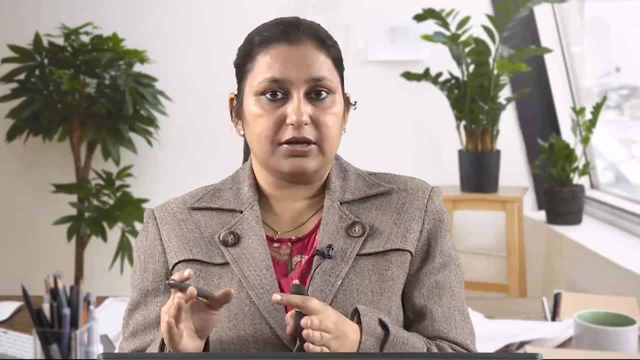 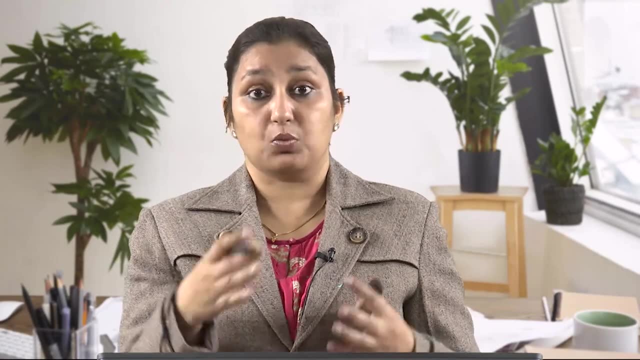 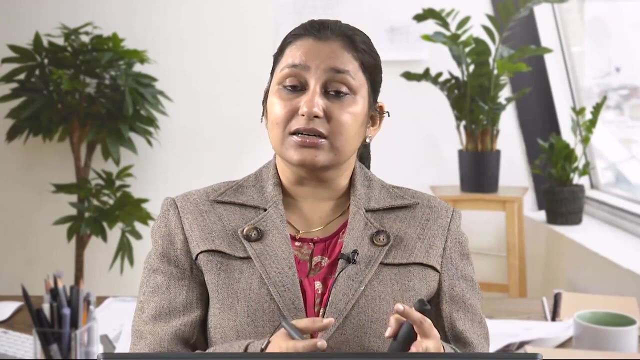 lot of these things Overall, even if you were to read a drawing without somebody explaining to you, should be able- one should be able to understand what is being said through a drawing, just like we understand a language composition. So you read a poem, you read newspapers, where? 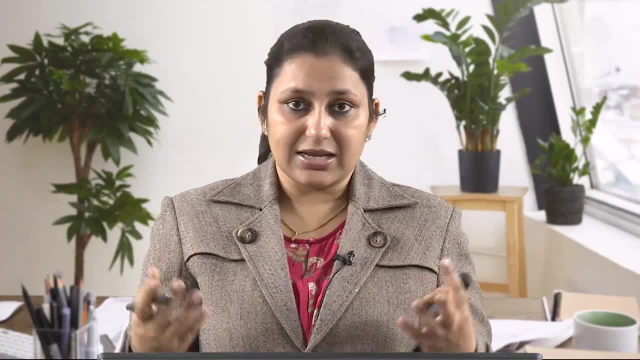 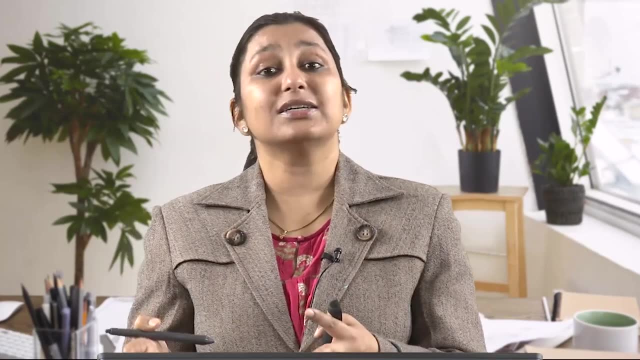 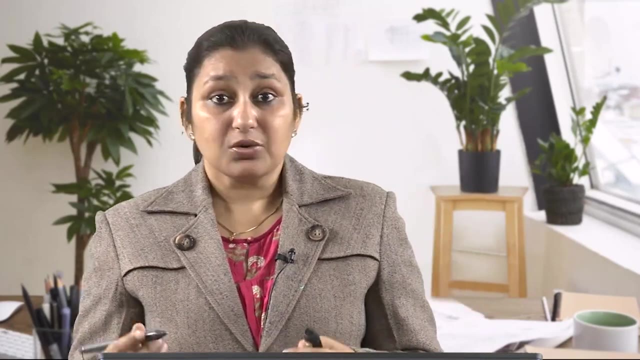 this communication is happening: Magazine articles, books, anything, just like. we read them and we understand what the author has been wanting to say. Similarly, we read a drawing and we understand what the architect or the engineer has been wanting to communicate. So when we talk about communication through, 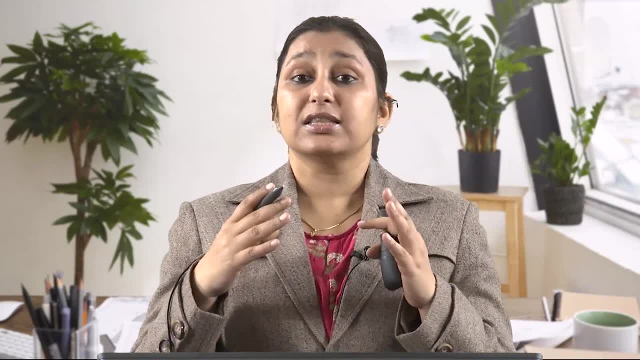 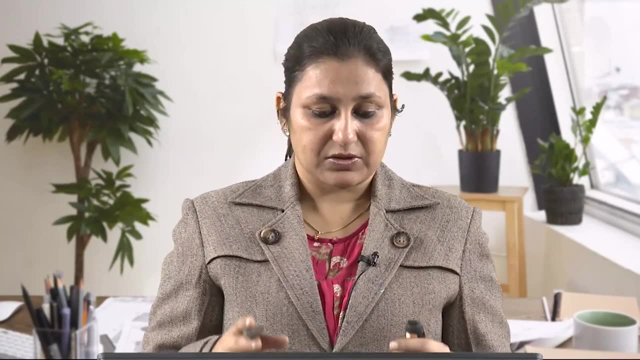 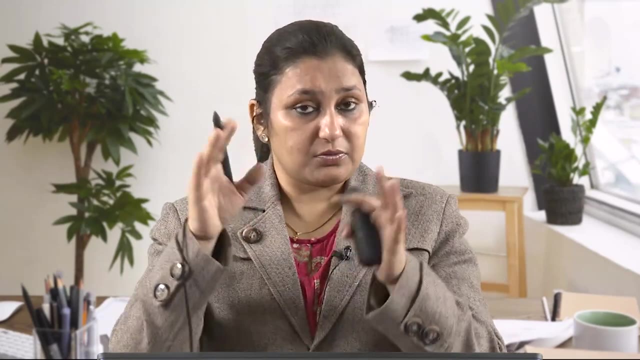 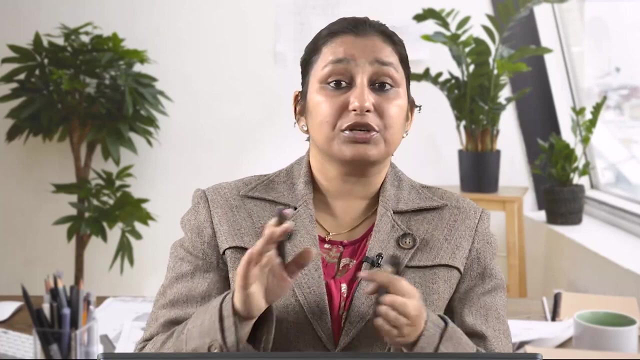 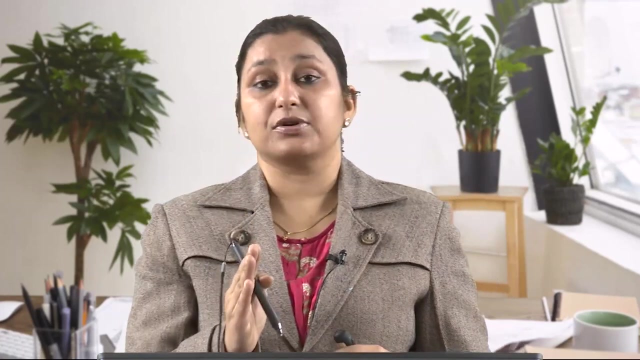 graphics. we are essentially talking about the communication of an idea, a design, through this medium which is graphics. It is the language using projections and there are different types of projections and, just like we are using these abbreviations and different words, we using these symbols as a standardized thing and, overall, it composes, it comprises of this language. However, we 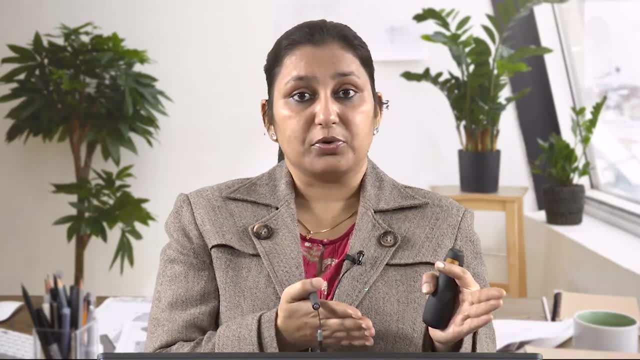 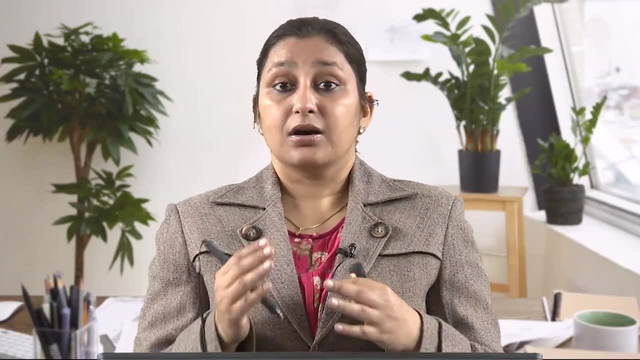 have to be very particular that, just like in general communication, we have a bad language. So sometimes if we do not use, choose a word, So we have a bad language, and sometimes we words carefully- it might communicate a wrong thing. you know it might communicate a wrong. 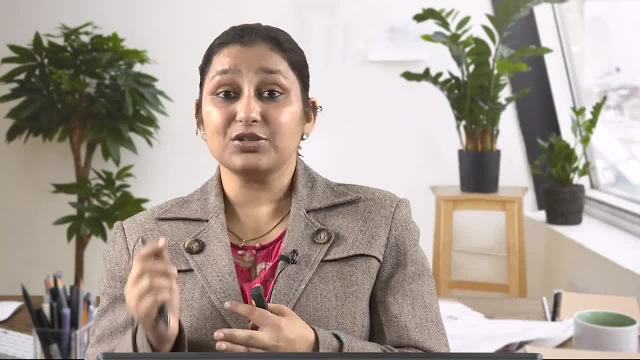 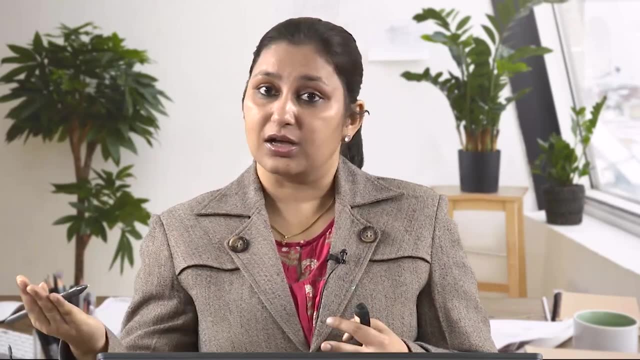 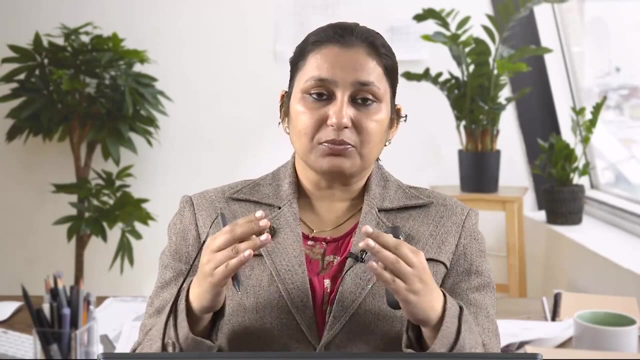 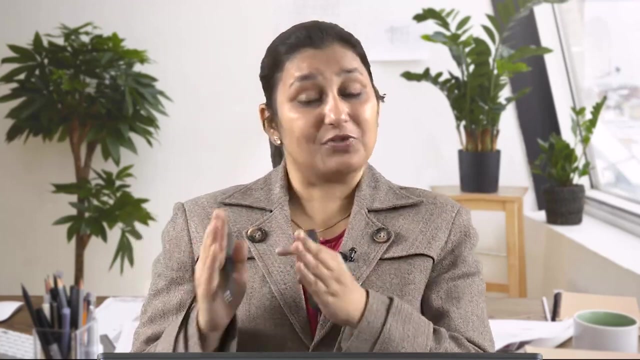 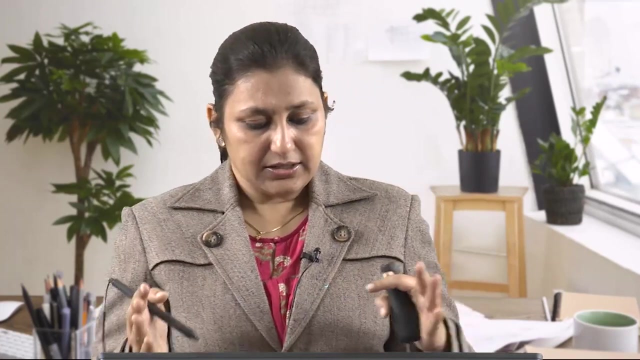 message. Similarly in drawing also. if we do not choose our lines, our symbols carefully, it might communicate something wrong and we might go ahead with a wrong design. we might just go ahead with something completely different being designed and constructed, So similar to communication. we have to be very careful of this language of design communication. 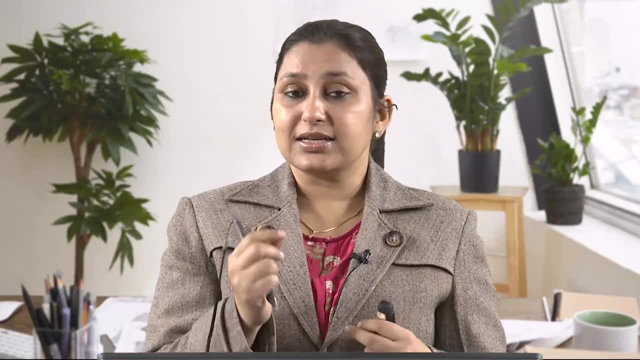 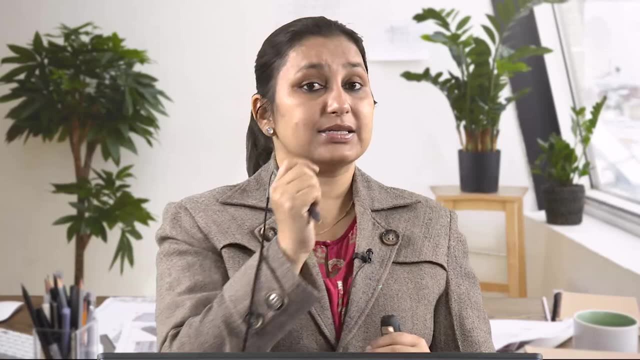 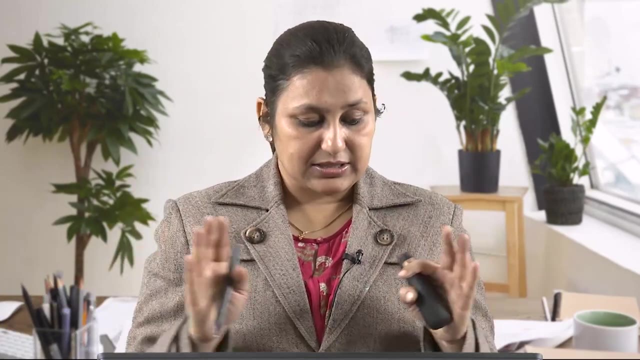 And how to standardize this. So when I say that ok, fan is represented in this fashion. So this is a standard symbol for fan, this is a standard symbol for ventilator, this is a standard symbol for window. These standards, they have been maintained through various national and international. 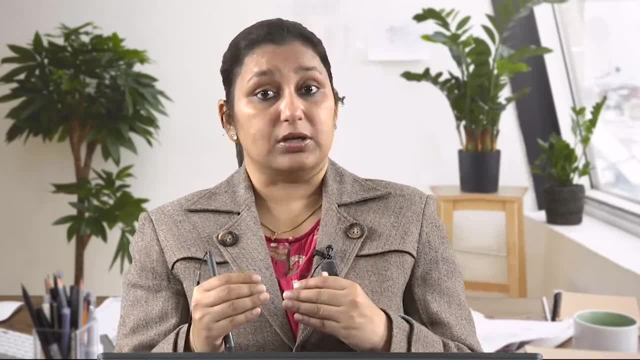 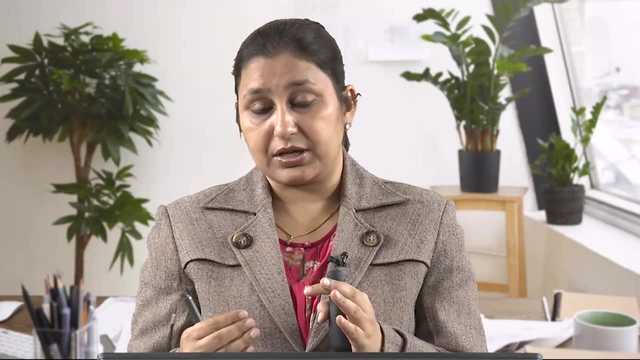 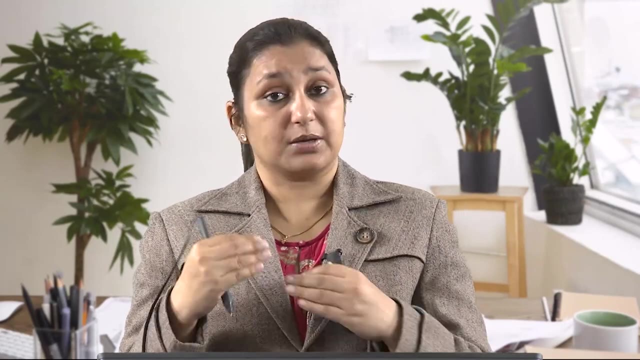 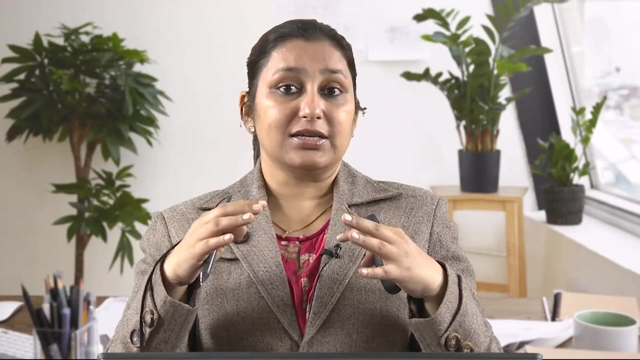 codes of practice. ok, and this is quite old, ok. So it started around the time when industrial revolution was happening and after that, specially during the world war times, this language of graphics, this communication through graphics, it flourished, But initially it remained. It remained confined as a military language. 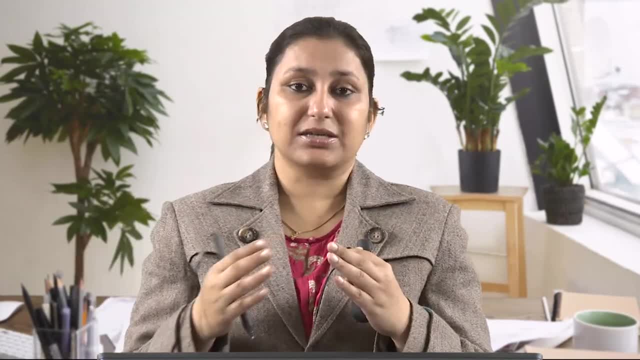 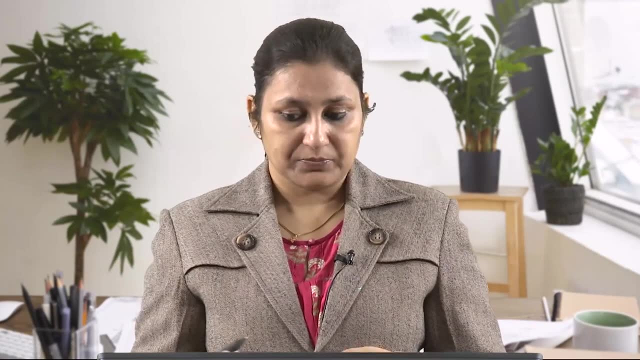 So it was not used commonly, but after world war 2, specially, it came out and it was used more and more by engineers and architects. So, if you look at, this is one of the drawings by Leonardo da Vinci and it is one of the 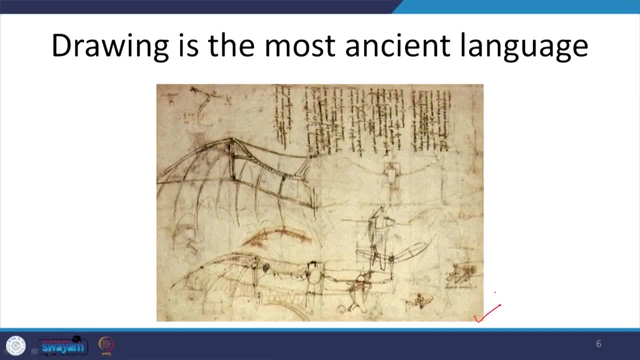 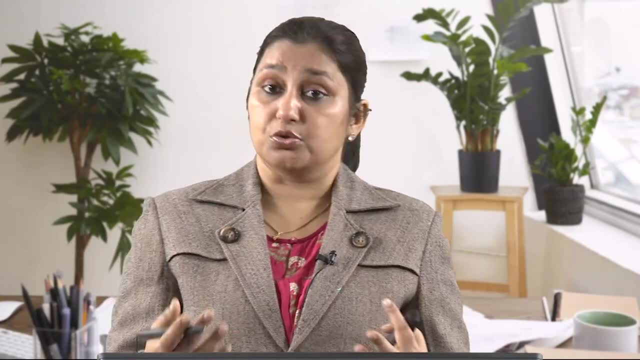 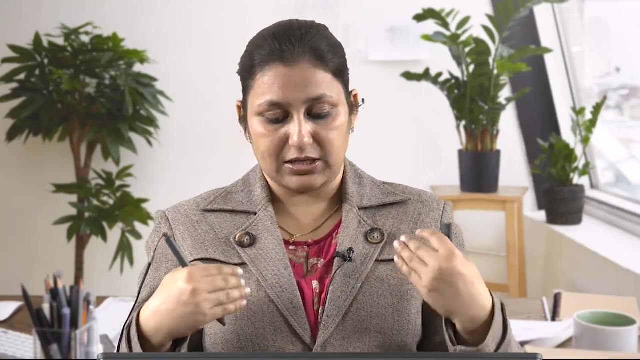 most ancient languages. Of course, Leonardo da Vinci is not a very olden times person, but he, if you ever get a chance to see how he drew. So this is his idea, his, you know, representation of the idea that he conceived, conceptualized. 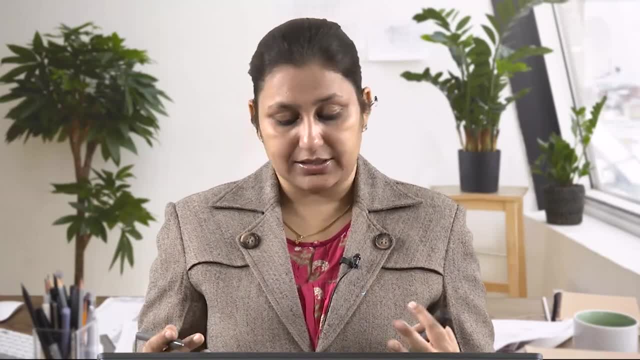 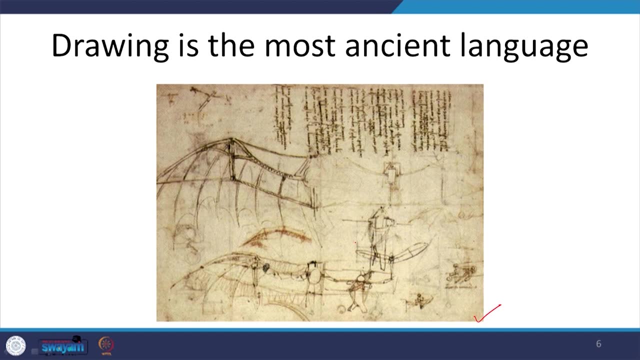 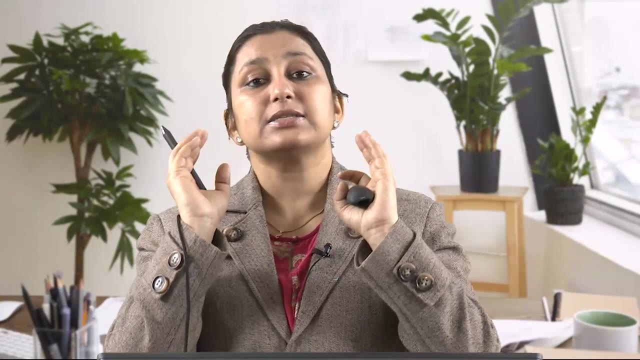 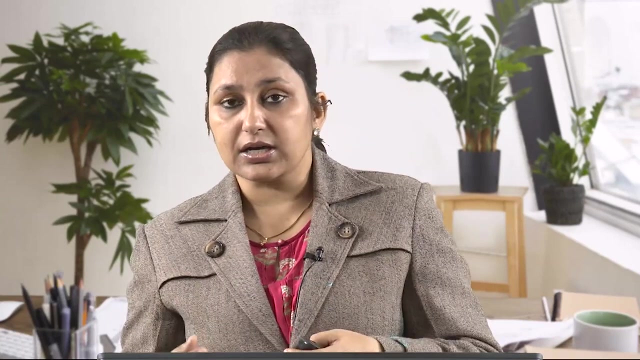 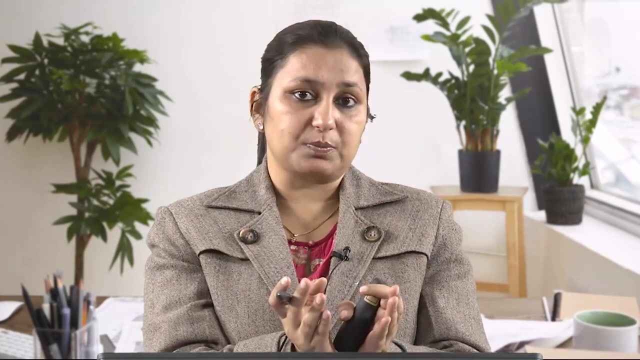 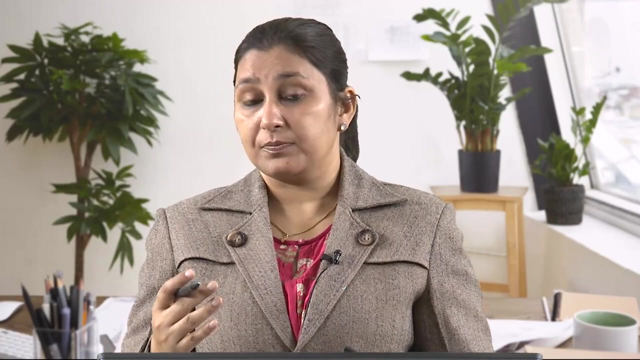 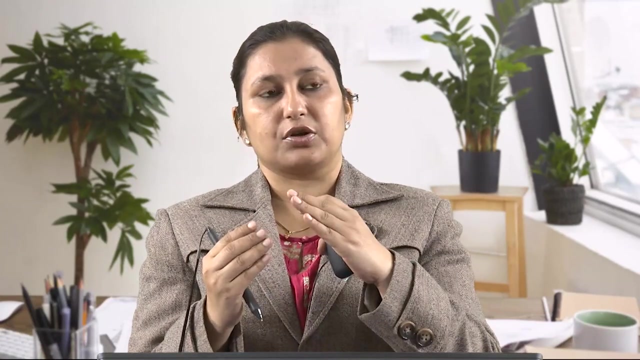 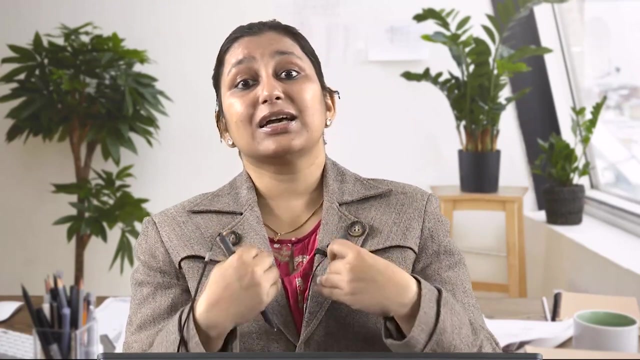 for a flying machine, basically an airplane, So based on the wings of a bat. So he was inspired by the wings of a bat and he was trying to convert all of this, you know, design, into a workable thing, The idea that, okay, I can paint and I do not really need to materialize it in a physical 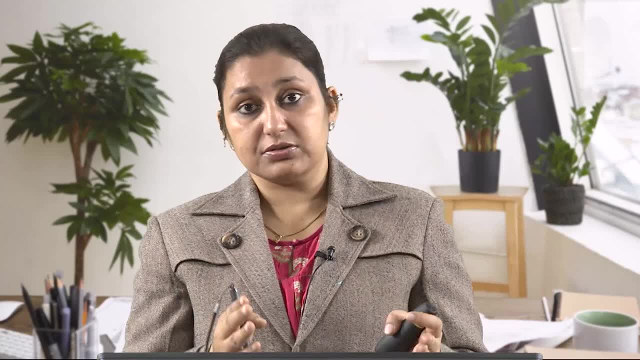 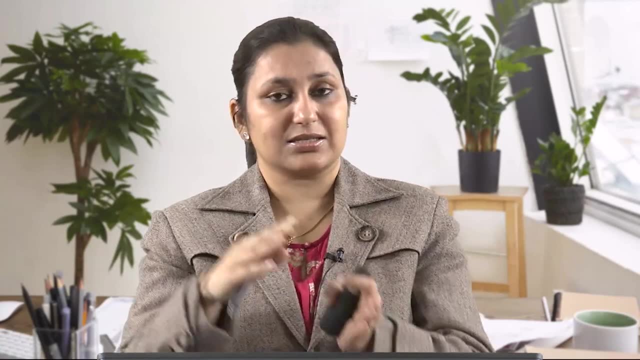 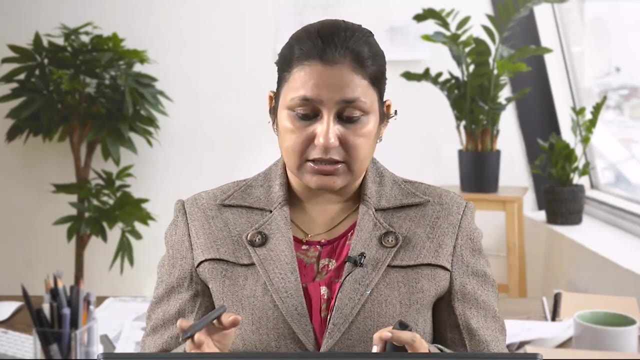 form. but when we are talking about graphics- engineering graphics or architectural graphics- we are really looking at conceptualizing this idea, materializing this idea in a physical form. So if we look at the need for graphics in engineering and design, we see that design process. 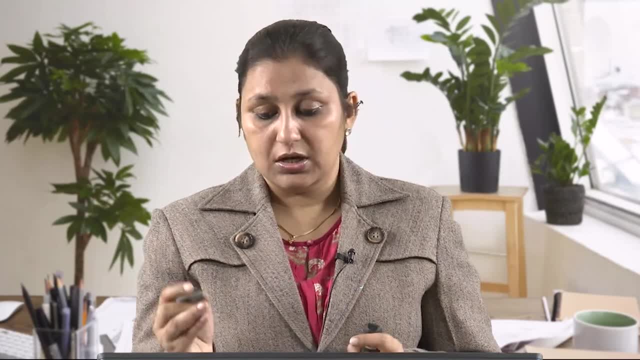 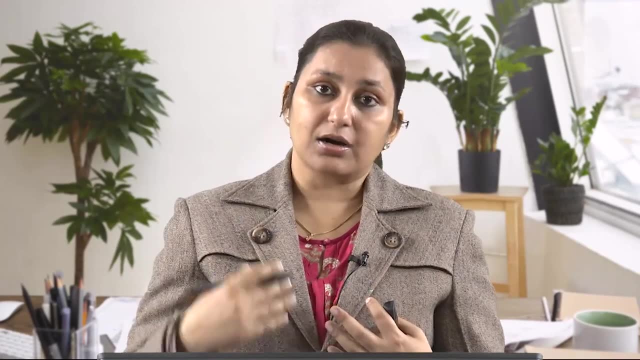 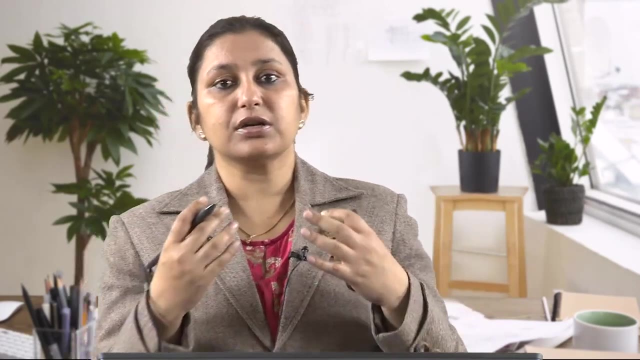 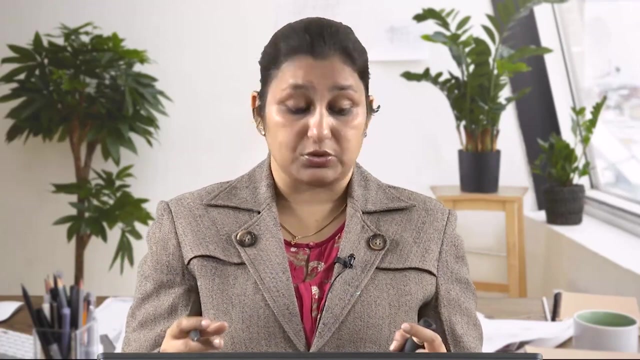 It does not always include the graphics skills it has to. without understanding this language of graphics, we will not be able to communicate our idea to the other person. So we cannot always tell, and even though we are communicating in general, the language of general communication, we cannot communicate to the other person what we really want to. 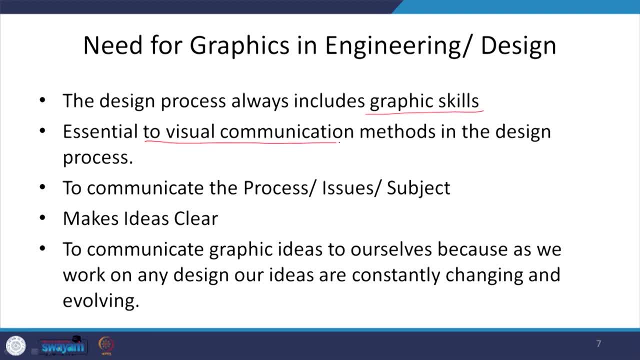 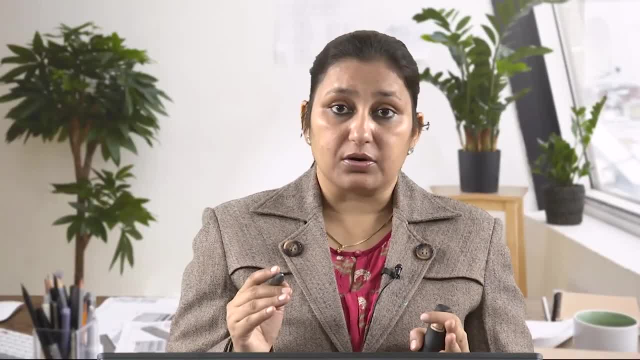 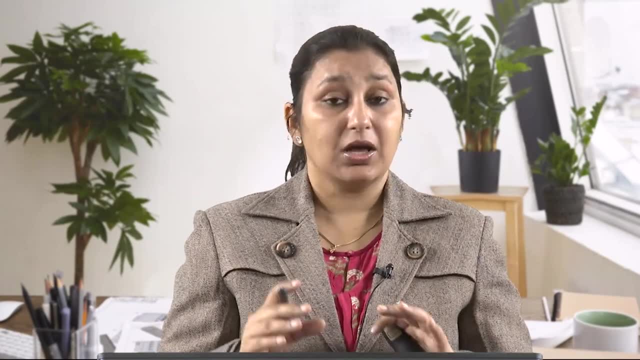 design. So it is essential to visual communication methods in the engineering methods, in the design process. So engineering graphics or architectural graphics is used to communicate the process or issue or subject whatever is being discussed, and to make that 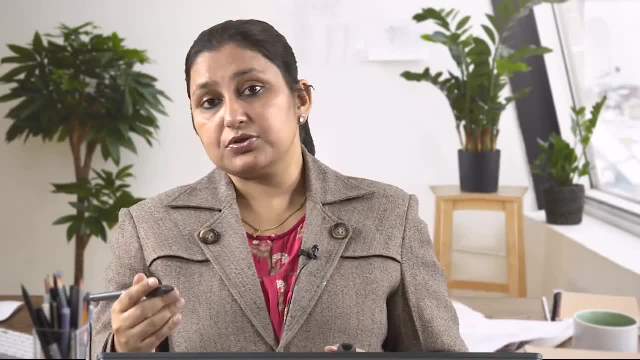 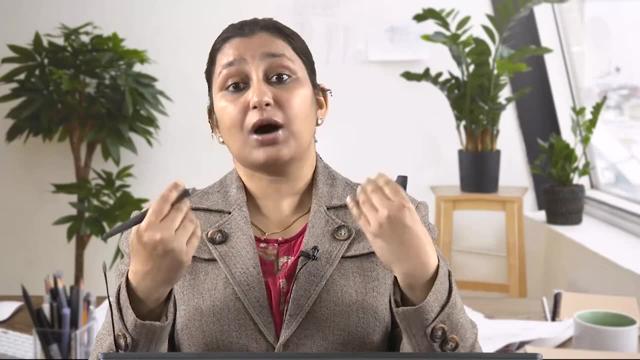 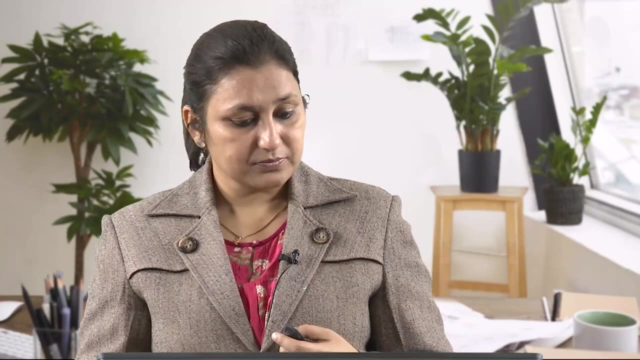 idea very clear, And not just for the other person, but also to ourselves, as we go on to design, as we go on to draw. it makes things even clearer to us who is drawing that how it is going to progress, how the idea is going to progress. 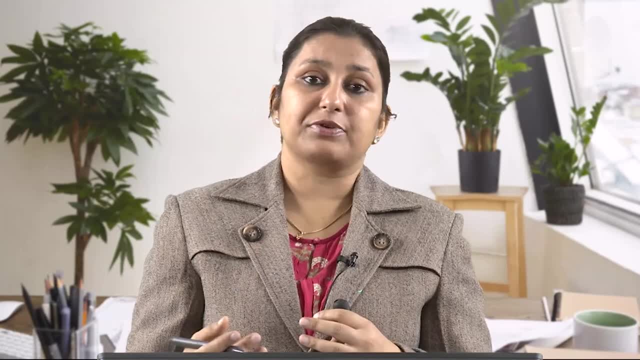 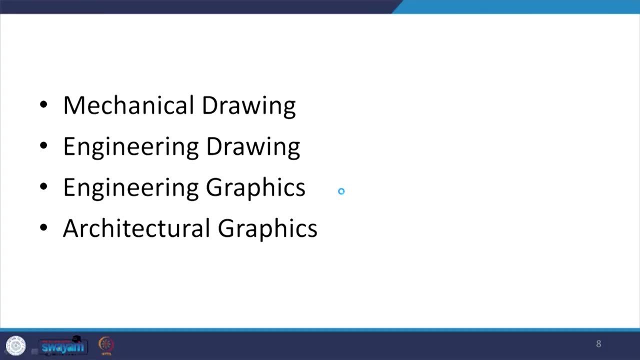 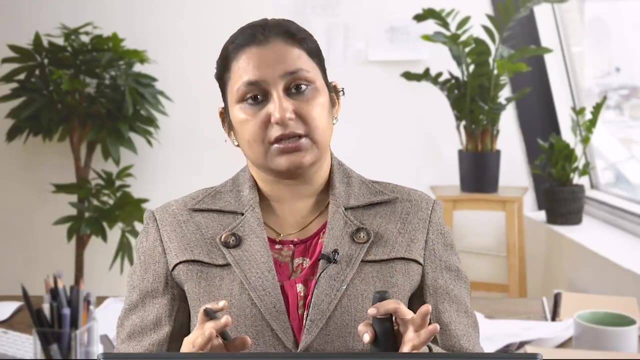 So what I call as engineering graphics or architectural graphics is also known as mechanical drawing or engineering drawing, or you could also find it in the name of engineering graphics. All of these they mean the same thing and they have more or less similar content. if you talk about architectural graphics, So you might be dealing more with the symbols. 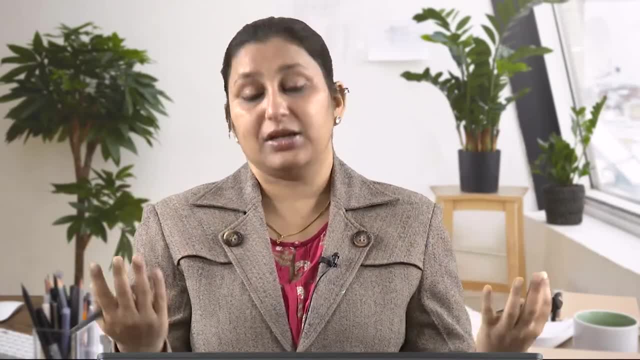 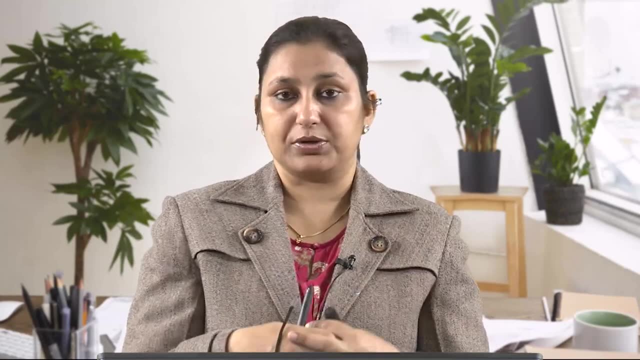 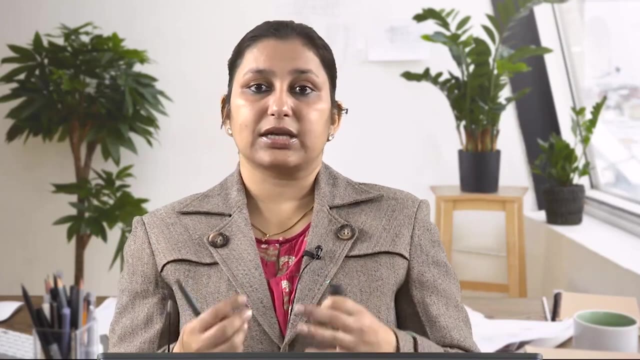 which are used to represent Different parts of the building. for example, the wall looks like that, the ceiling would be represented like that, a window would be represented like that. However, if I am talking about engineering graphics, where an engineer is using it to design die or nuts or bolts, 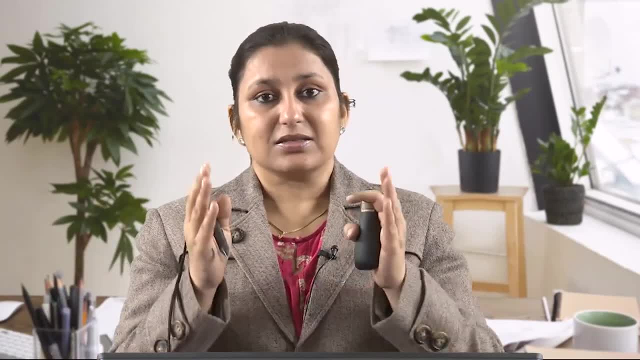 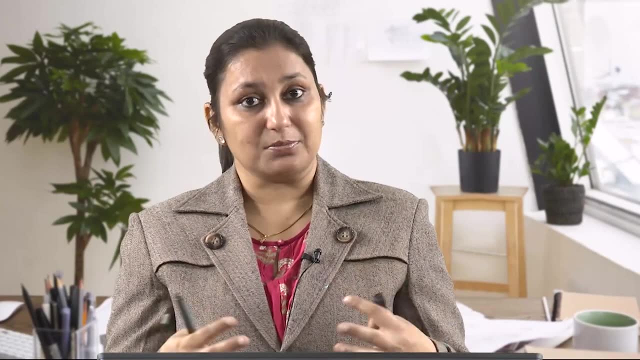 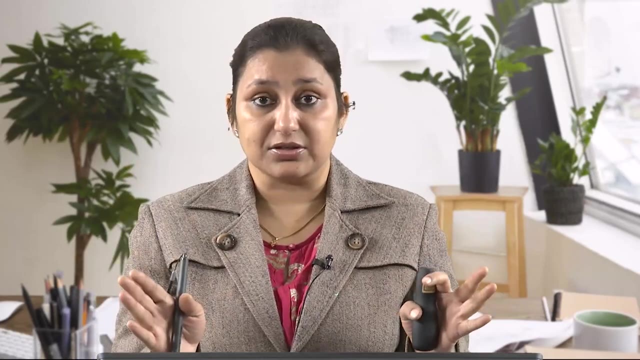 or different machines. the language will remain the same. the graphical language will remain the same. It is just that the symbols which are being used, mostly Popularly, for communicating that particular idea will be slightly different, though they are standard. So if a nut is represented as something in engineering graphics, it will be represented. 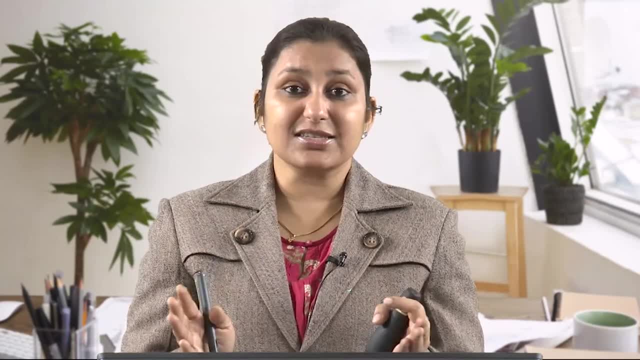 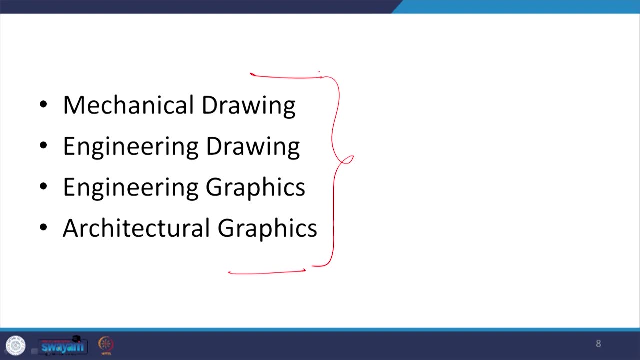 as exactly the same in architectural graphics as well. It is just that it is not being used enough. So, in a sense, what I mean to say is: all these are the same things. It is the same subject. You could pick up any book for mechanical drawing or engineering drawing. 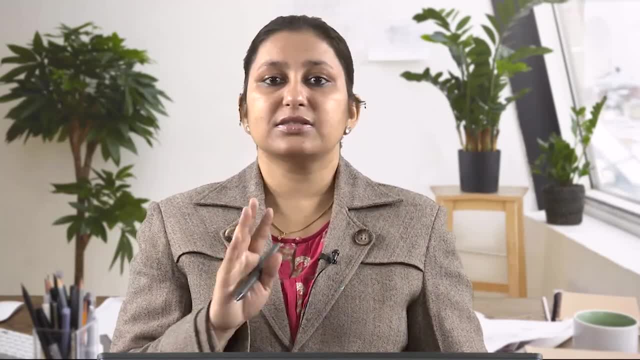 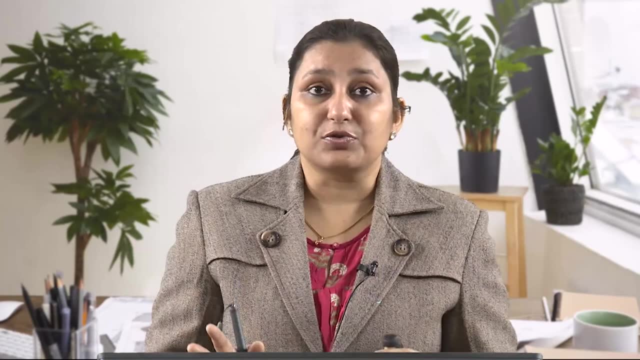 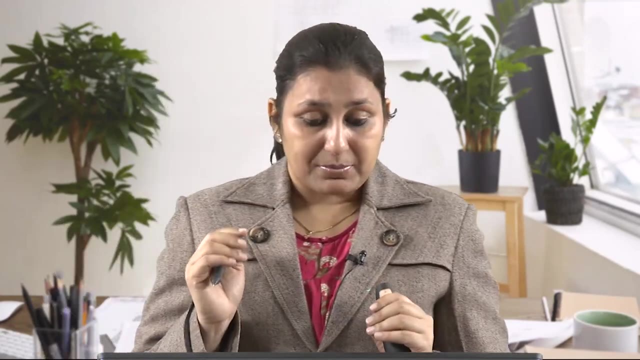 engineering graphics or architectural graphics, and you would find the same fundamentals being discussed, especially when we are talking about orthographic projection. So what is the difference between a sketch versus a drawing? and I think I have somehow some way discussed this, But a sketch is basically just representation of an idea which is 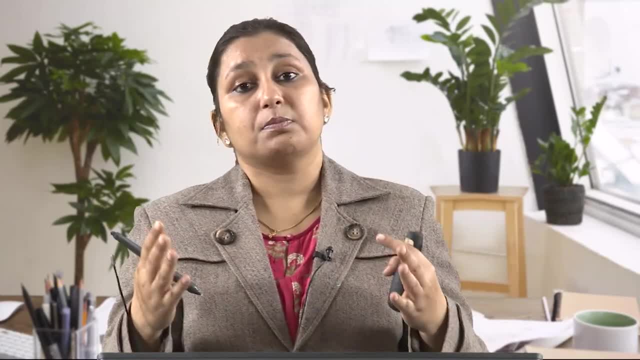 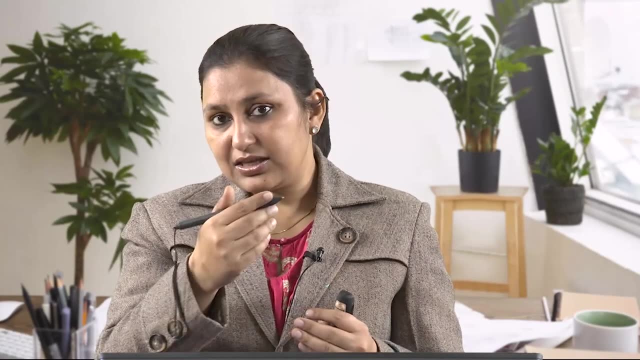 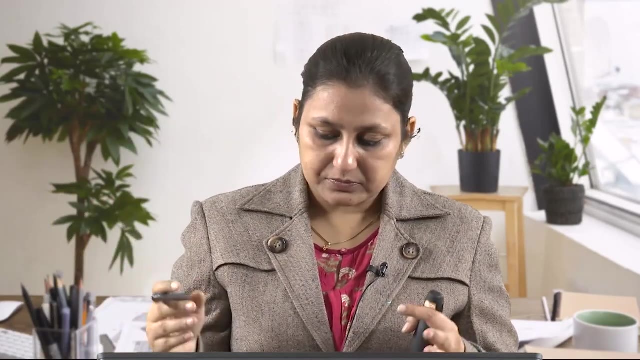 in our mind. So if we looked at the drawing which was made by Leonardo da Vinci which I just showed, So it had a sketch like thing, and then by the side it also had a drawing with some little dimensions on it. So a sketch is a representation of an idea, but it is. 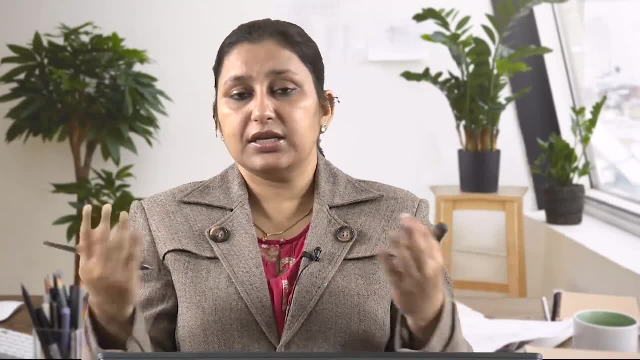 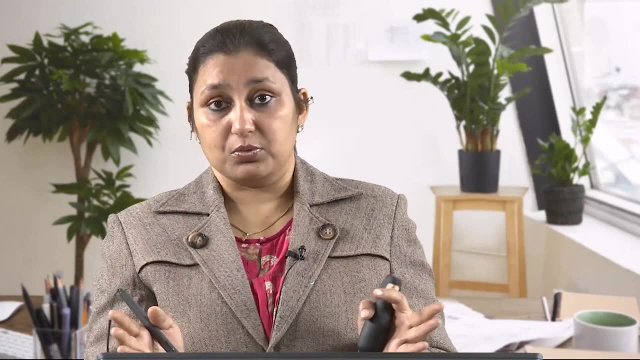 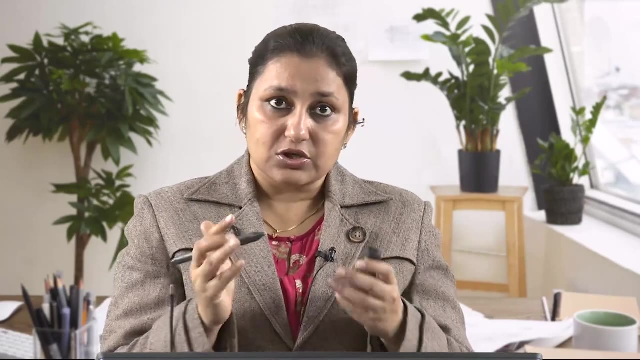 quite ambiguous. Any different person can understand it in a different way. However, the drawing is absolutely unambiguous. It will convey only one thing. It will convey one thing. It will convey only one thing. It will convey only one thing thing, and that is what it is supposed to convey. So, sketch, while could be conceived, perceived as 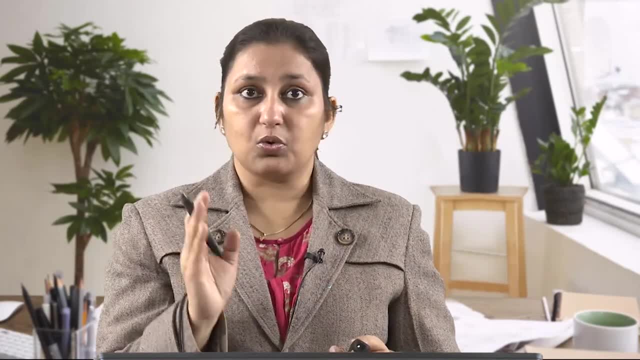 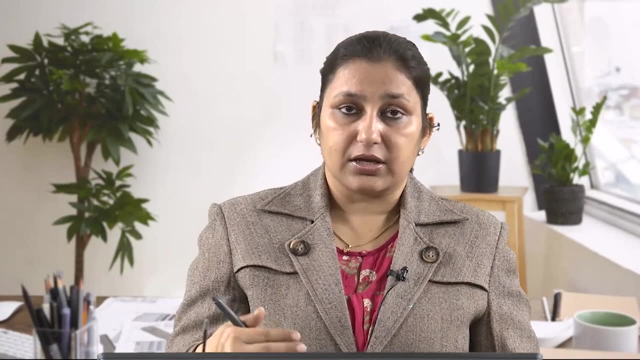 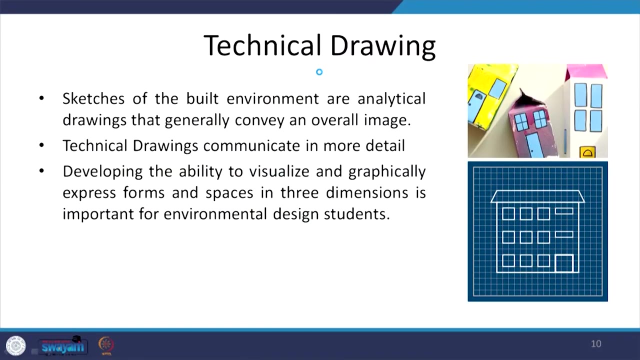 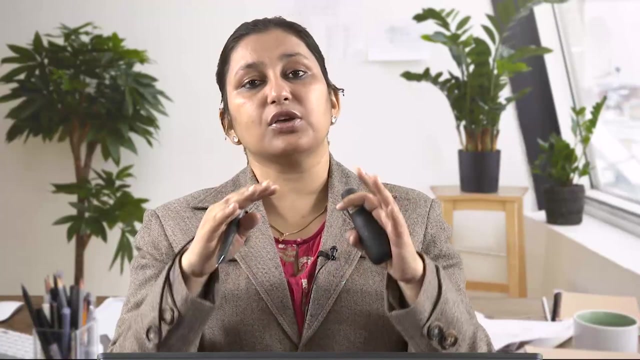 different by different people. drawing cannot be. Drawing will only convey one meaning. So, within drawing, when we come to this technical drawing, we, and especially when we are talking about this architectural drawing, it is the sketch of a built environment which, along with the analytical drawings that can very clearly convey the overall image of this building. 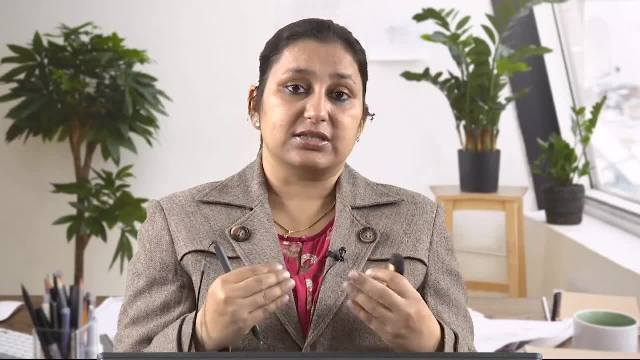 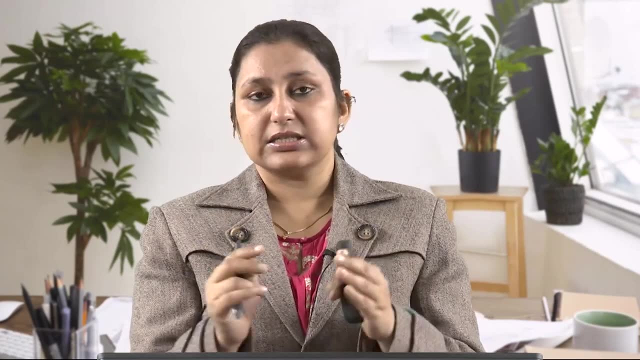 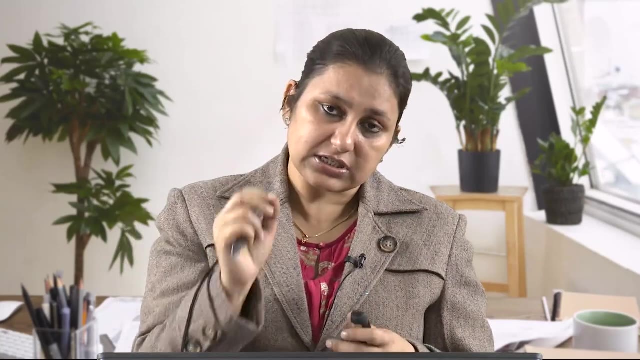 The built environment which is in question, which is in discussion, which is being designed to be constructed tomorrow. So they have all the details: the dimensions, the measurements, the different types of materials which are going to be used. It has utmost detail which will be required to design it tomorrow. 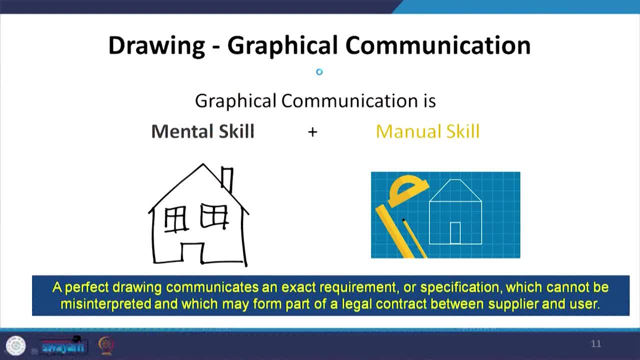 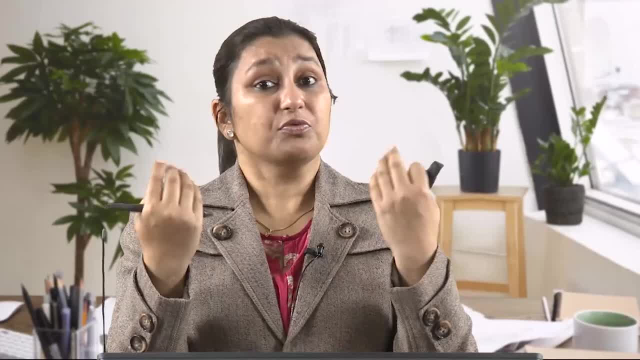 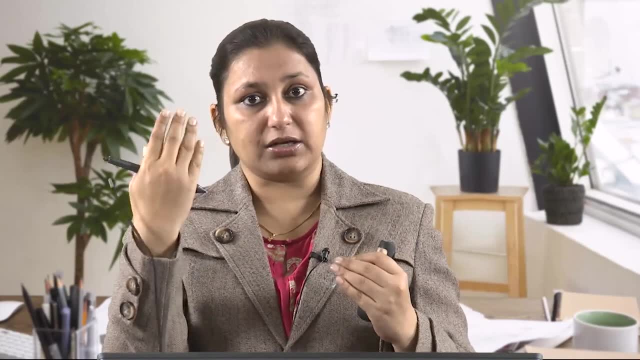 So when we are talking about this graphical communication, we are basically looking at both the mental skill- So you have to perceive things, you have to be able to visualize, imagine what is going to happen- and then manual skill to translate all that imagination onto the paper. 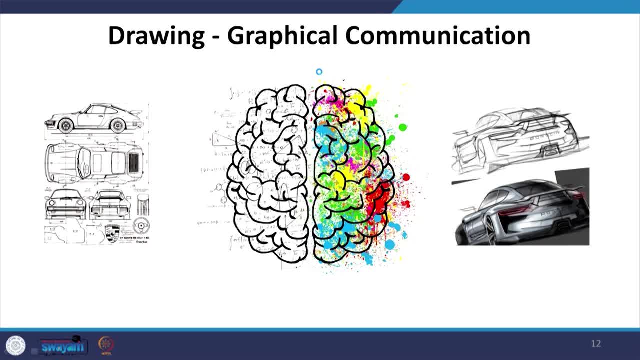 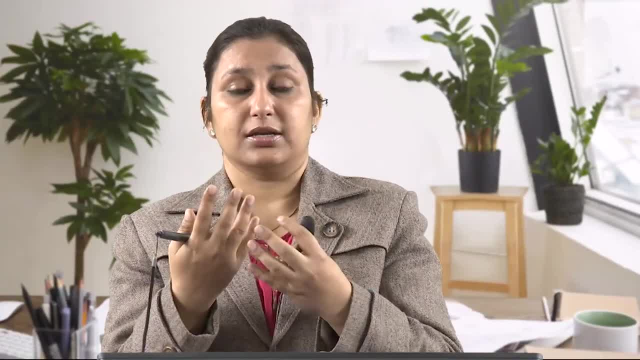 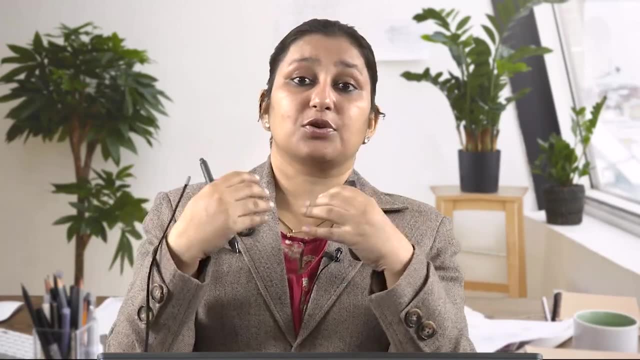 So it is putting both of these things together, It is using both sides of your brain, basically. So on one hand, we are imagining what we are wanting to design. say, a building, a house in mountains is what we are designing. So I just visualize that this house is going to have. 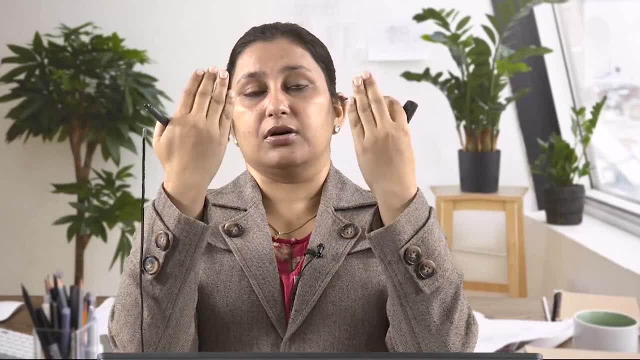 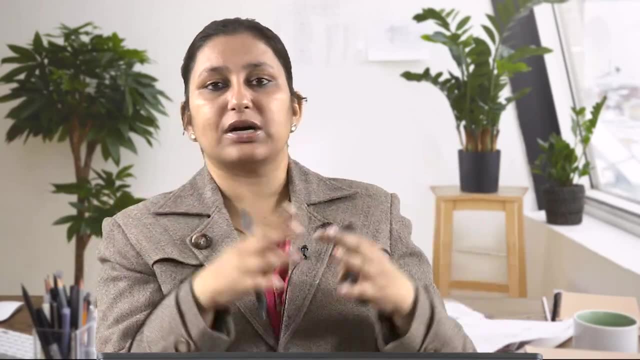 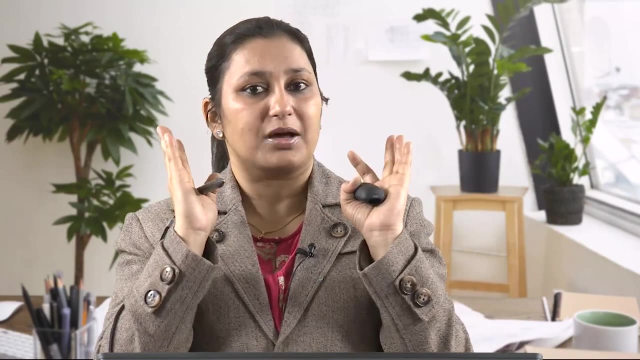 a lavish big balcony and it will have a sloping roof and it will have a wooden column and it will have very huge, vast windows. As I say all these things, I have a certain picture of this house in my mind. I know what I am imagining is this kind of house. 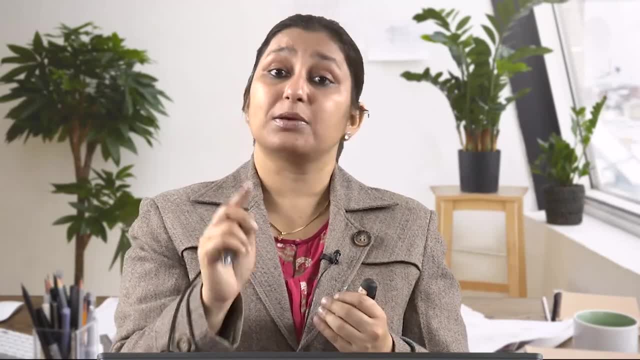 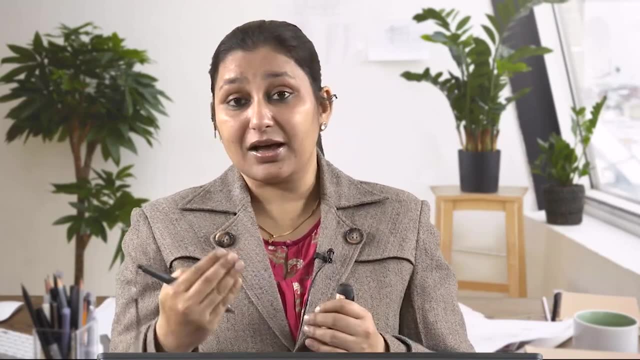 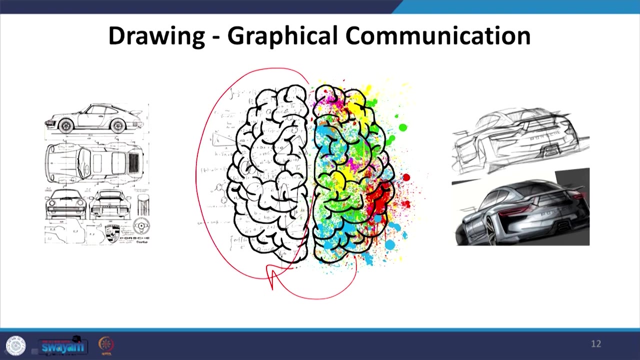 While you are listening to what I am saying, you are also imagining what this house could be. The moment I start, I have to get it constructed. I will have to convert this creative idea into a design, a drawing, which is analytical. So it is not just that okay. 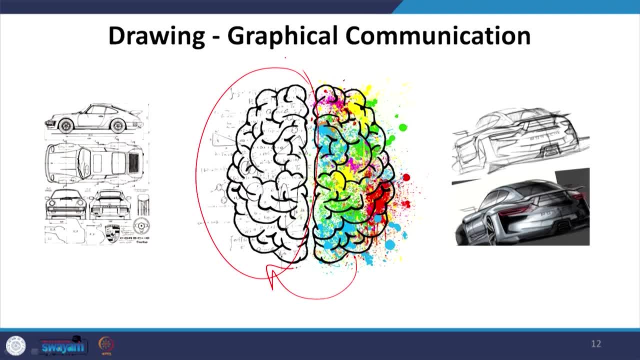 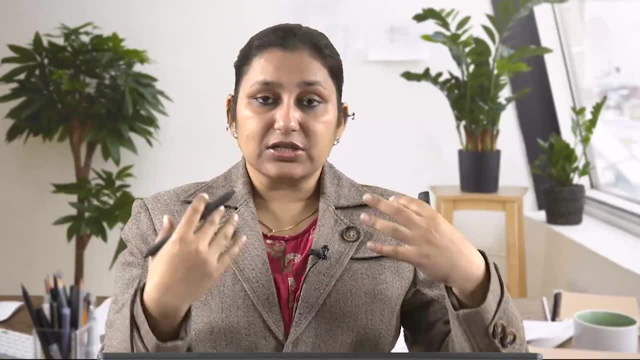 I cannot have any slope. I would have to know, okay, what size of the rafter would be needed, What size of the column would be needed to hold this beam and this rafter, what kind of you know material would go for the flooring, what kind of foundation would go? 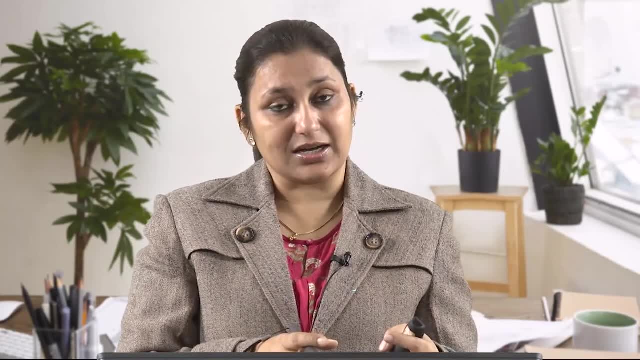 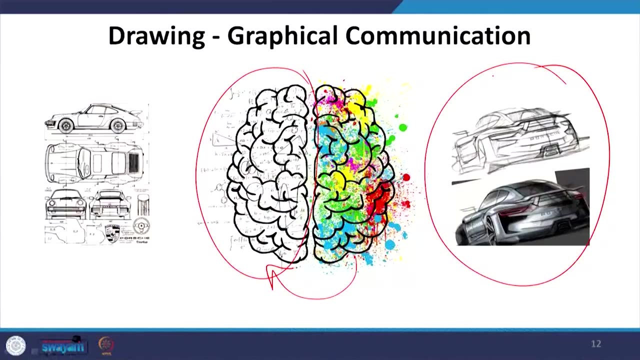 and I have to talk about all those analytical aspects of this design for it to actually so. this was my idea, for example, of the home here. it is a car and I have to actually make it like this, where I have all these individual dimensions, I have the materials and everything, so that this 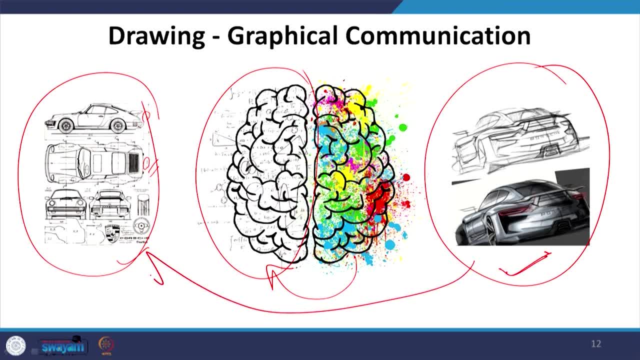 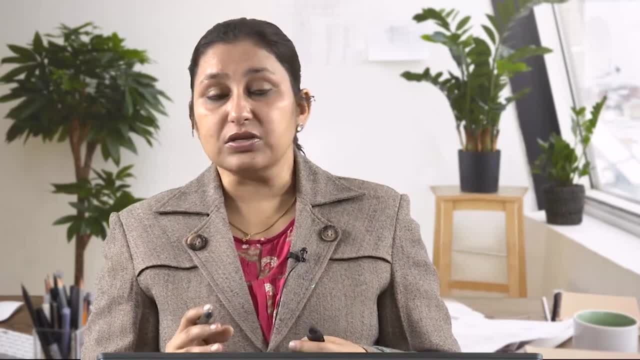 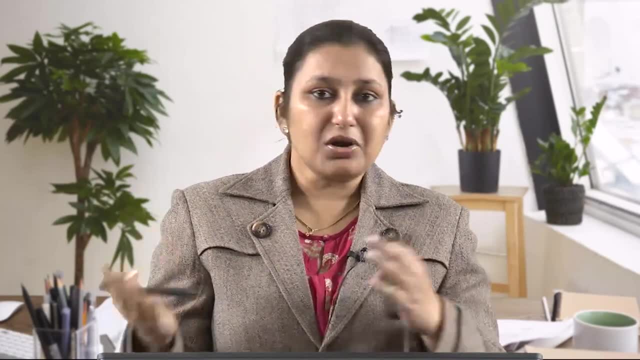 idea which I had in my mind be converted into a reality through with the help of these drawings. so that is what is the sole purpose of this graphical communication. now, when I say that it is a very standard drawing you cannot have, it would also mean this and that: no, there is. 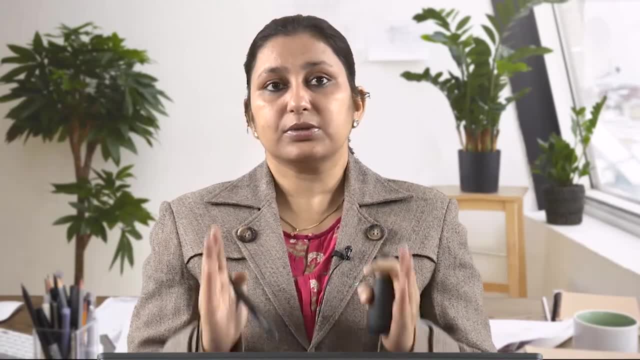 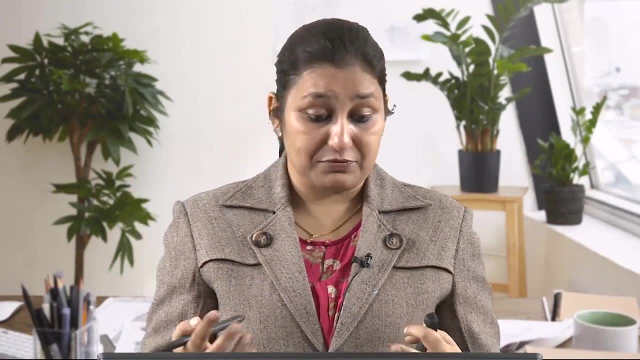 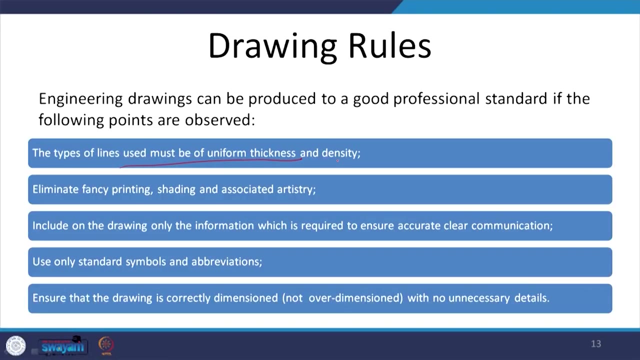 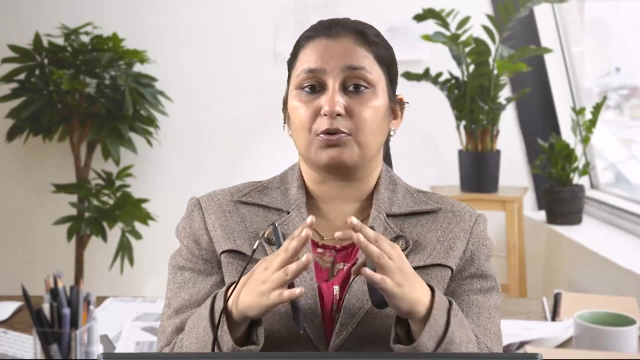 no scope for that. so there are certain very rigid rules when we draw these, when we make these drawings, when we go So, one that the lines that will be used they have to be of uniform thickness and density when we when we move the pencil. so things have been made much simpler with the help of these. 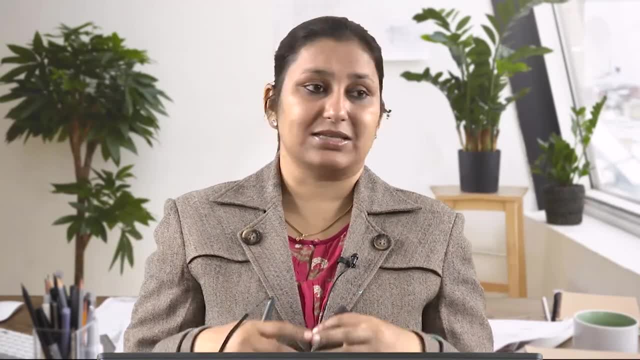 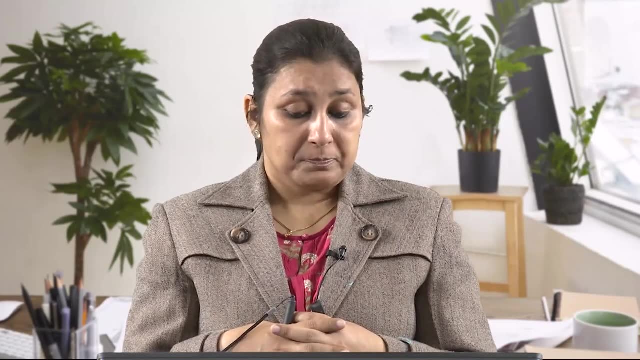 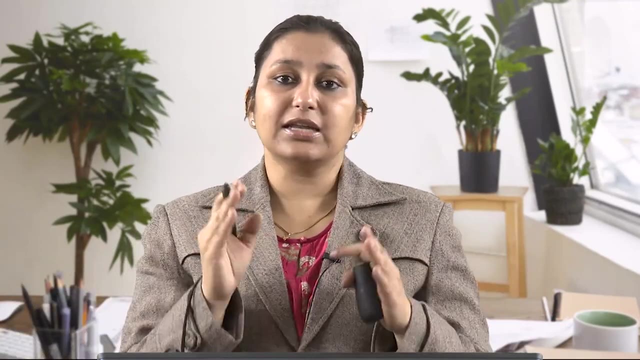 CAD software, computer aided drawing software, for examples. AutoCAD is there. you have, you know, many other softwares which are used to draw these drawings. So it is much easier. you select a line thickness and you draw a line of a certain dimension, certain measurement and 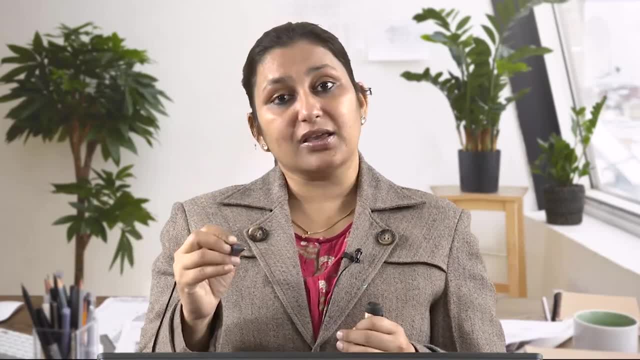 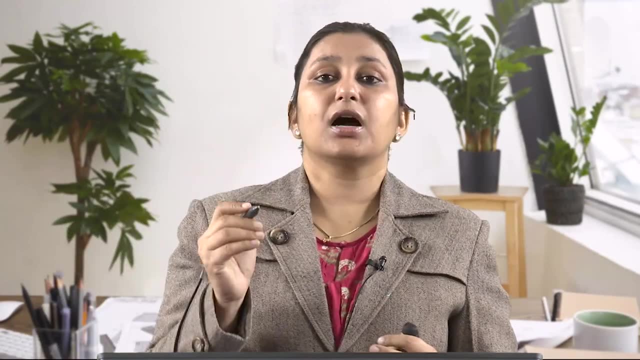 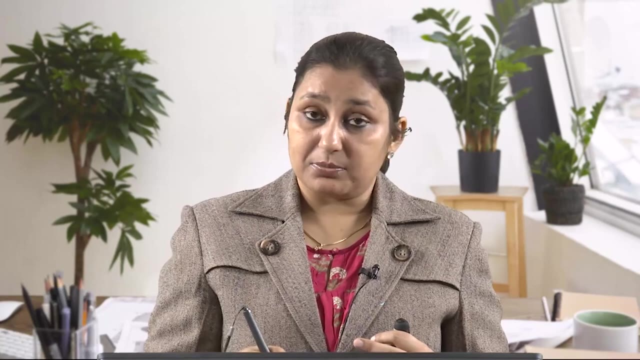 it will be absolutely uniform, but when the drawing was mainly done by hand and, by the way, in this particular lecture, in this particular course altogether, we are going to uh draw it by hand and you will learn how to draw it by hand. So that is why I m am emphasizing that the lines 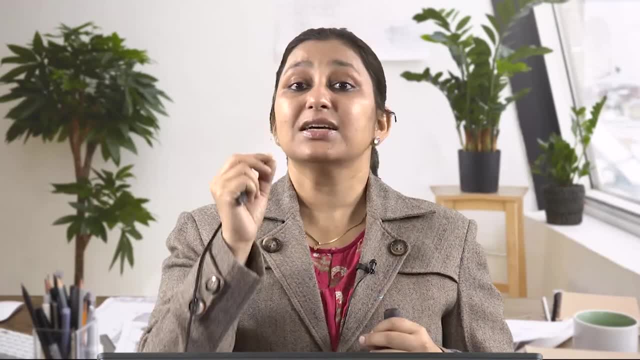 have to be of uniform thickness. in graphics, the variation in line thickness has to be of uniform thickness and the lines have to be of uniform thickness. In graphics, the variation in line thickness and the variation in line thickness is different, So this is the same thing You can. 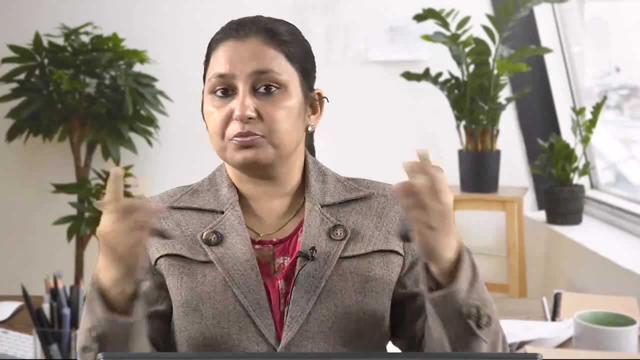 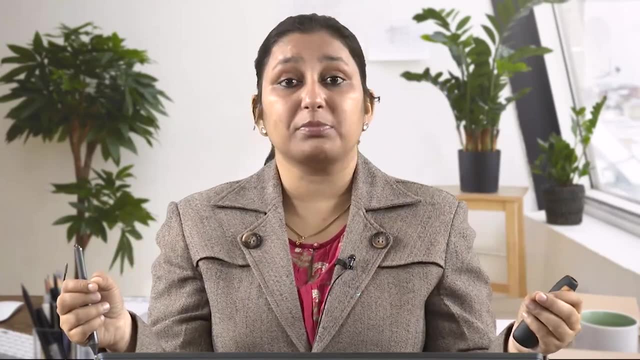 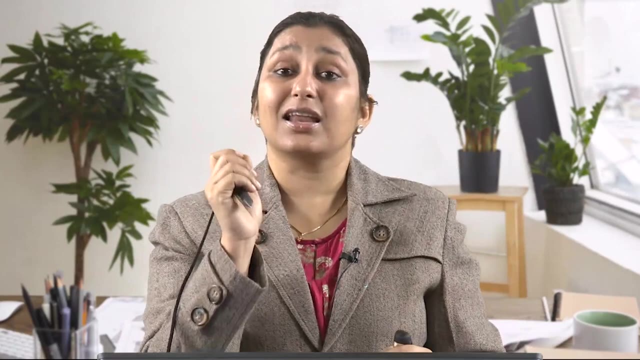 thickness also has different connotations, that it has different meaning. If I have to show a line which is being seen and plan, I will probably I will make it thicker. If I have to show another beam which is in the ceiling right above this, I will make it lighter. So there is a difference. 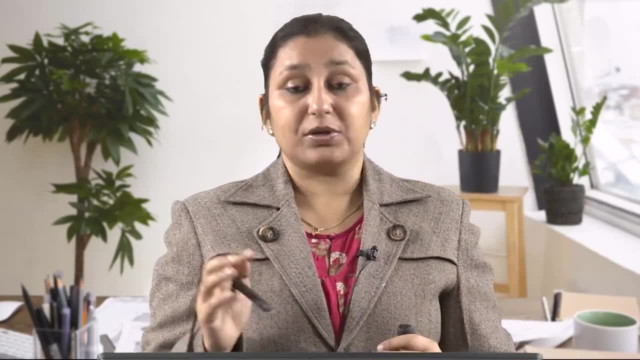 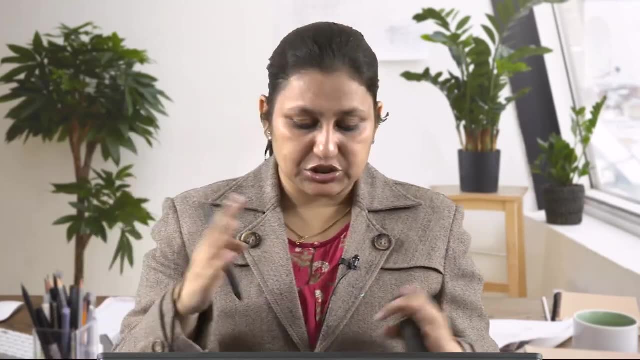 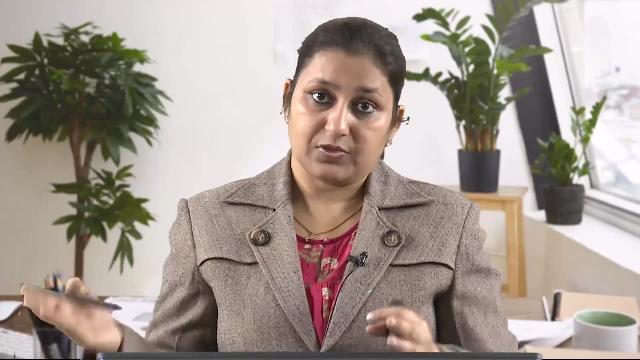 that is why when we use these lines, any line, it has to be of uniform thickness. We cannot use fancy printing and coloring and shading and associated artistry, because a drawing will be reproduced multiple times. For example, I have to design a space, a room, a hall, say. 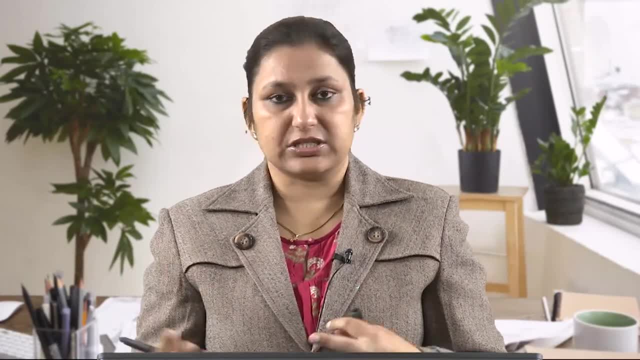 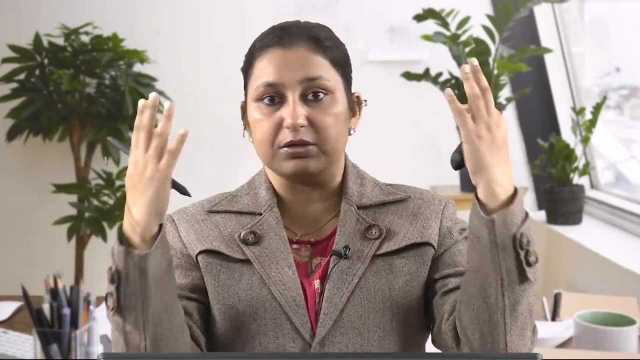 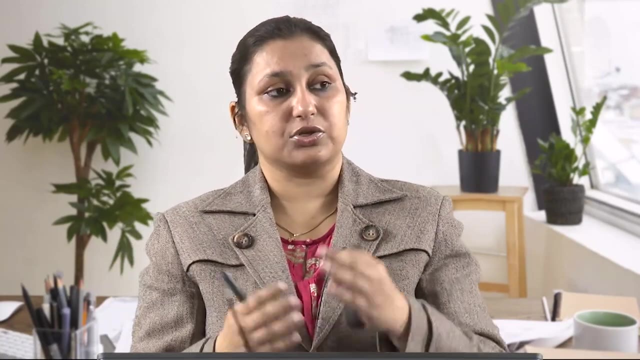 and there are multiple things which are going to be fitted in this room One. there will be these brick walls. So civil works will be there: walls, columns, beams, ceiling, flooring, everything. so they are the same set of drawing, with slight variations, will be given to the civil contractor. 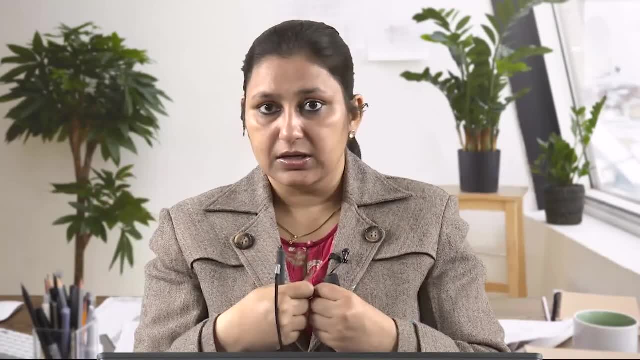 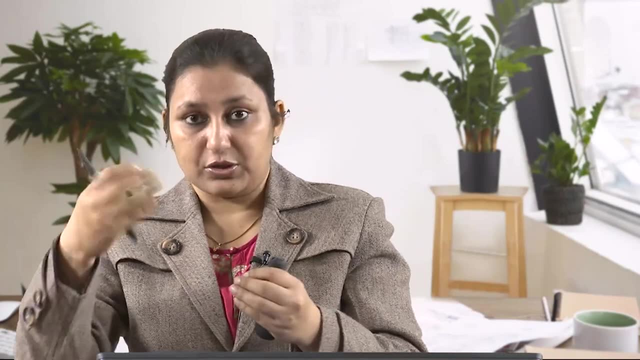 Then we have to get all these electricity works done. So there will be lights, there will be fans, there will be conduits running. The same thing has to the same set of drawing with, of course, additional information related to electrical will be going to the electrical contractor. 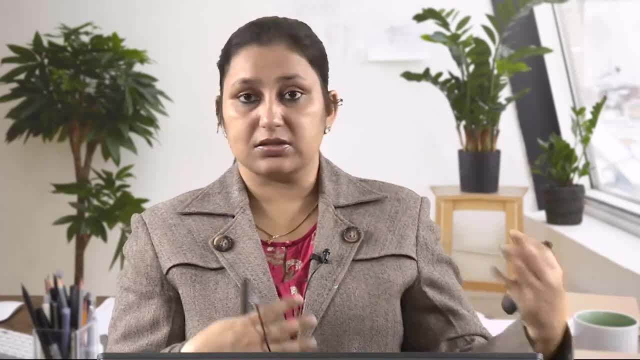 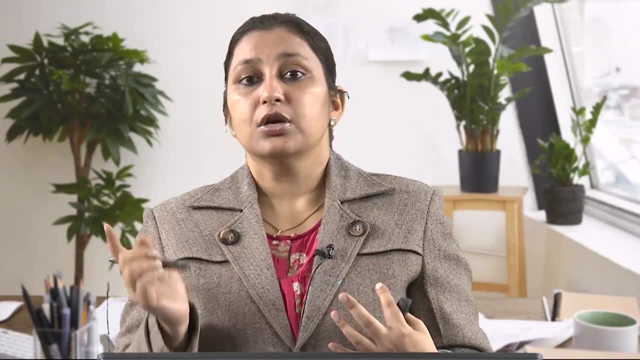 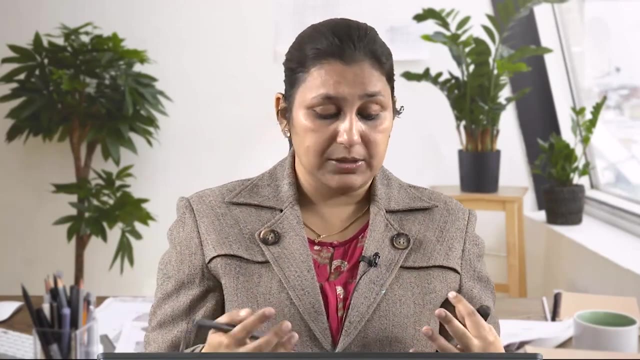 There will be another set, probably the mechanical one, the plumbing, the, this, that furniture guy, So. So everybody will be using this drawing and it has to be reproduced. So we cannot put colors, it will produce shades and it can be perceived wrongly. 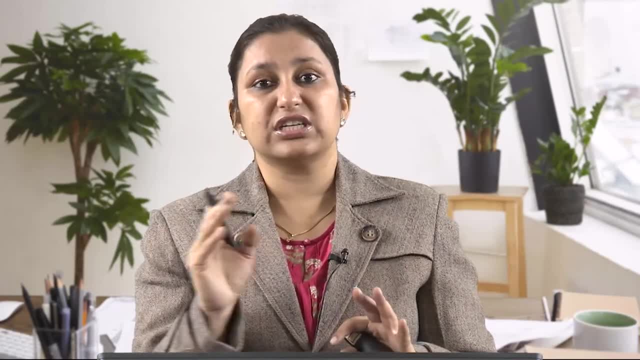 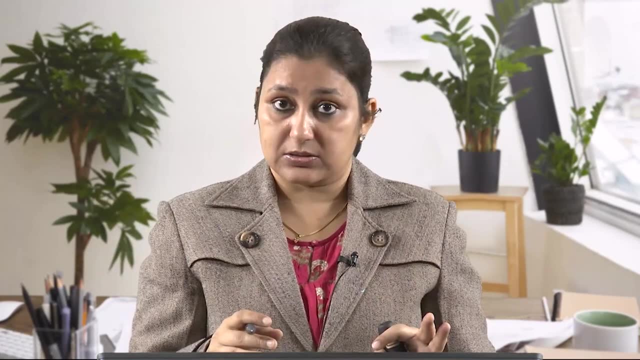 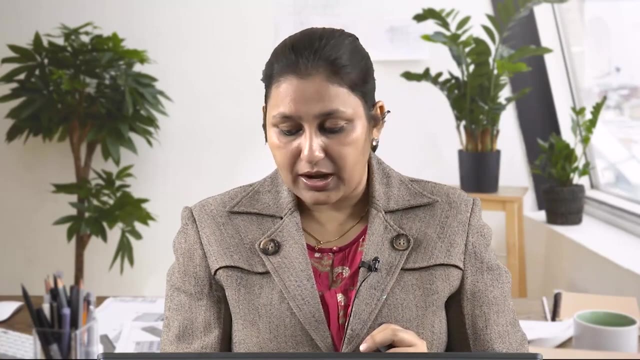 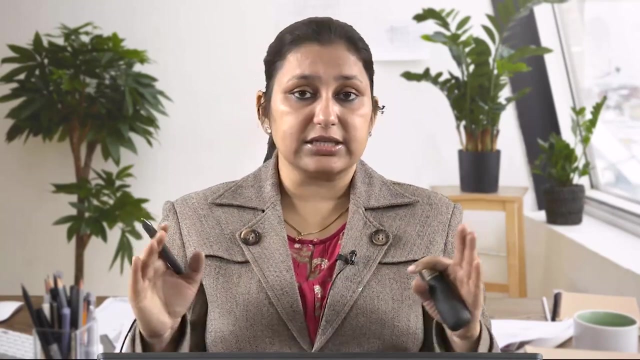 So we cannot have any color printing, shading or any artistic representation on engineering drawings. The next: we have to include only the information which is required so that the communication is absolutely clear. So we should not include anything which is not needed in the drawing. 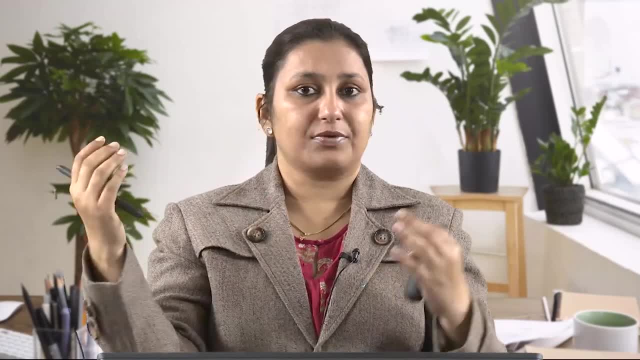 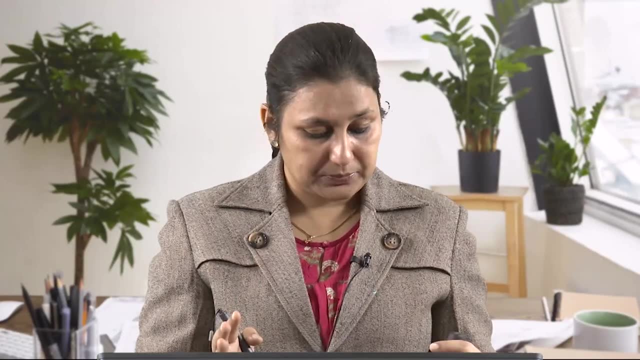 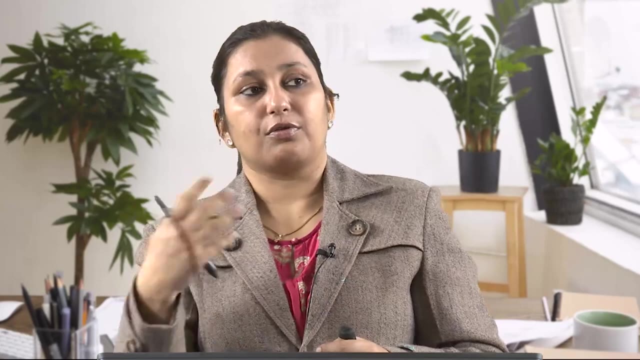 So only the necessary ones. we cannot have unnecessary, irrelevant information added on the sheets. It is very simple and it is very clear And we use only standard symbols and abbreviations. So the standards, as I said, for representing fan or light or any plumbing accessory, everything. 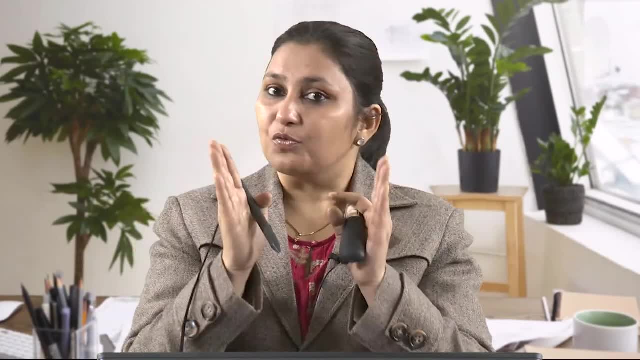 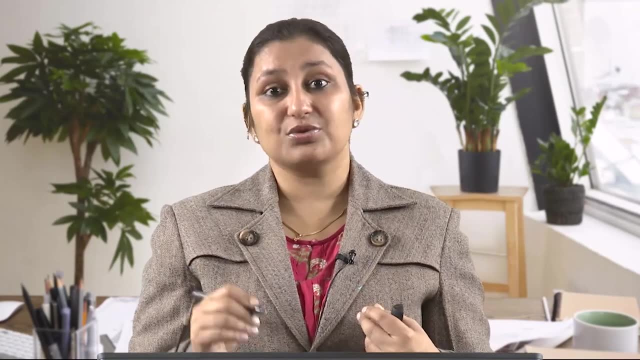 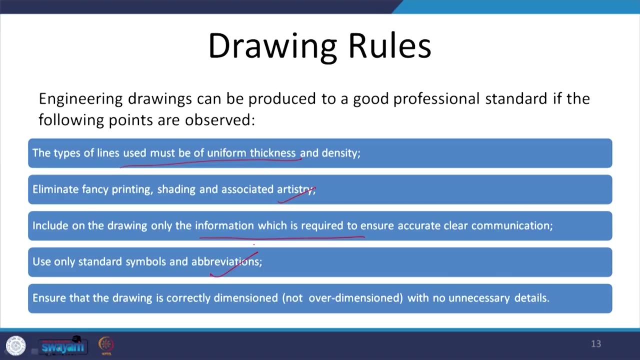 has a standard symbol and there are abbreviations which will be used and it will only be read that way. So we have to know what those standards are, what those standard abbreviations and standard symbols are and the same be used. The next we have to ensure 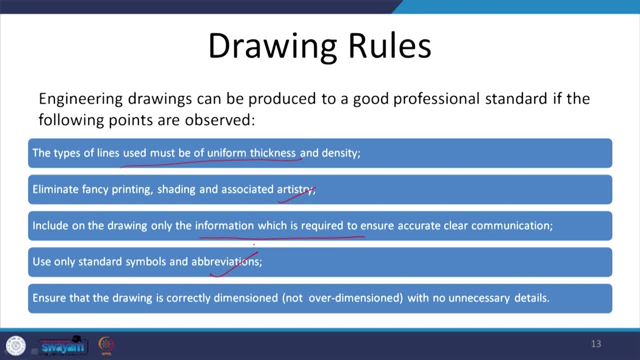 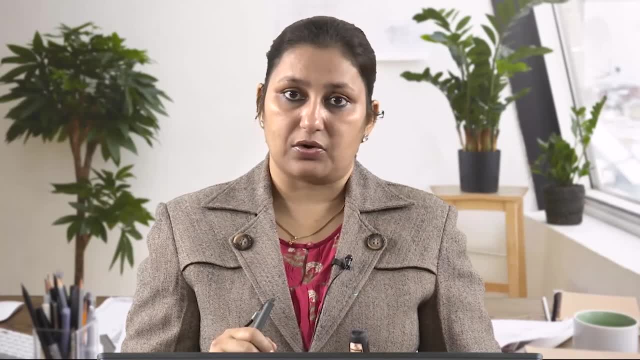 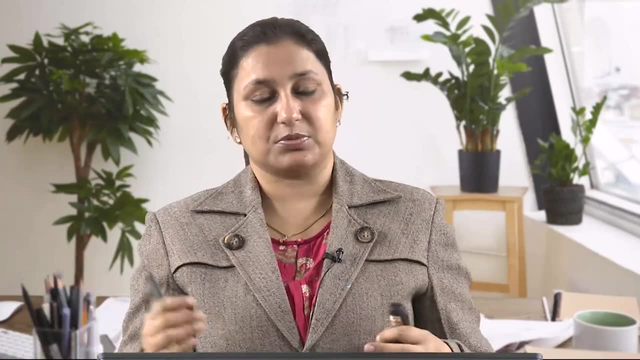 that the drawing is correctly dimensioned, with no unnecessary details. So a drawing is almost meaningless if it does not carry a dimension along. I might make a room, but if I do not know what will be the size of this room- 3 meter by 6 meter or whatever- it will have no meaning it. 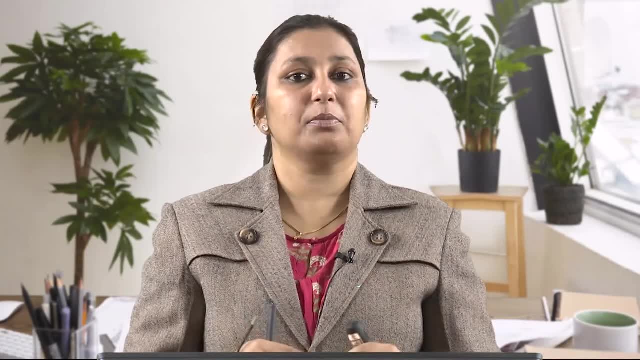 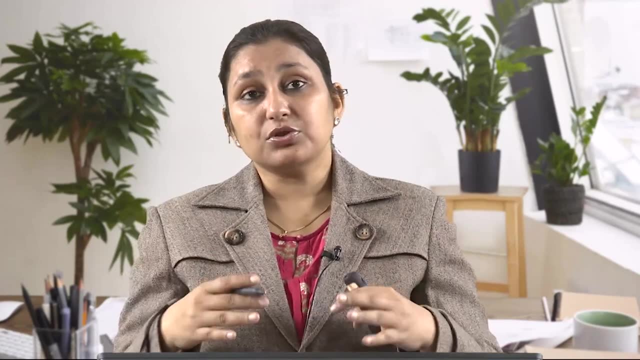 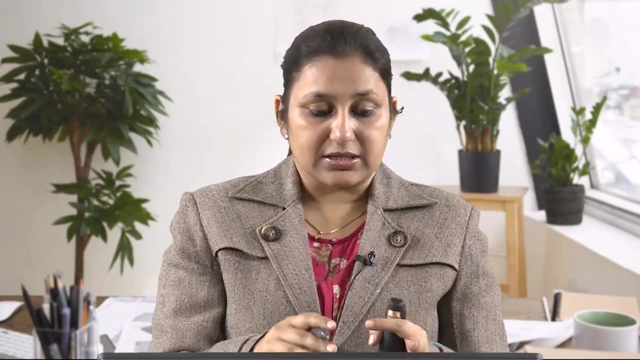 cannot be constructed, So it always will come, should come, along with dimensions and, of course, the scale to read it. So if we come to this, almost the conclusion of this introductory lecture, I will conclude it by narrating, by telling you the qualities of a good drawing. 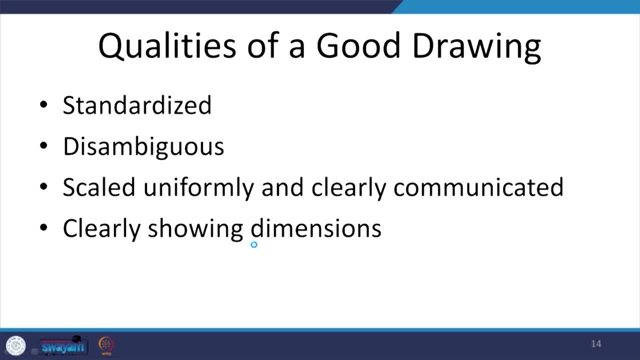 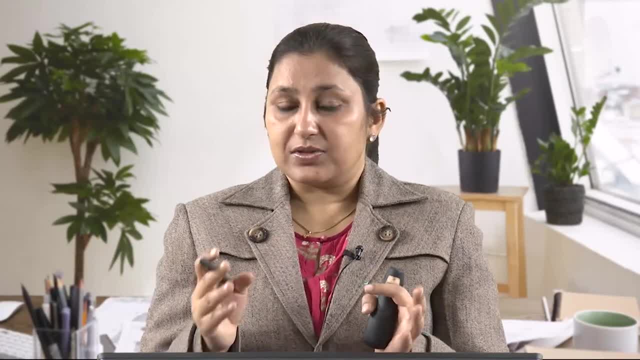 When do you know that the drawing is a good drawing? When it is a standardized drawing. Are we talking about architectural drawing, engineering drawing, So it has to be standardized. The symbols, the representations used in the drawing have to be the standard ones. 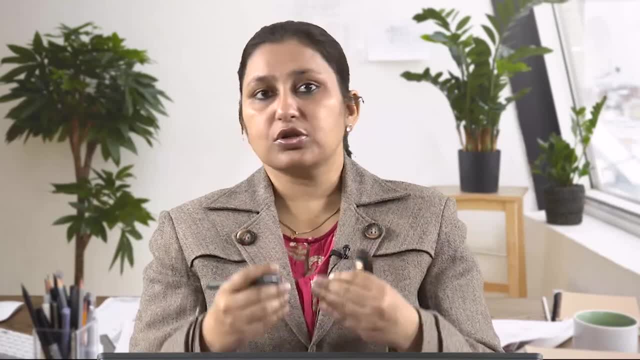 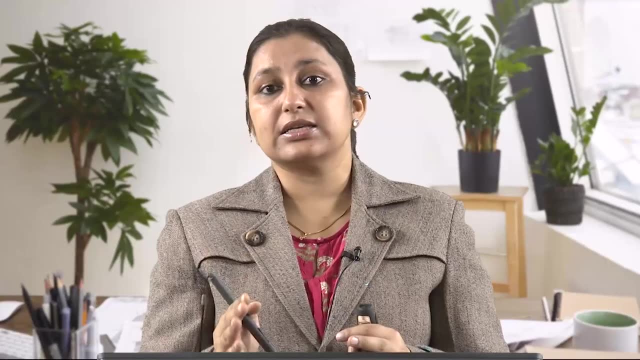 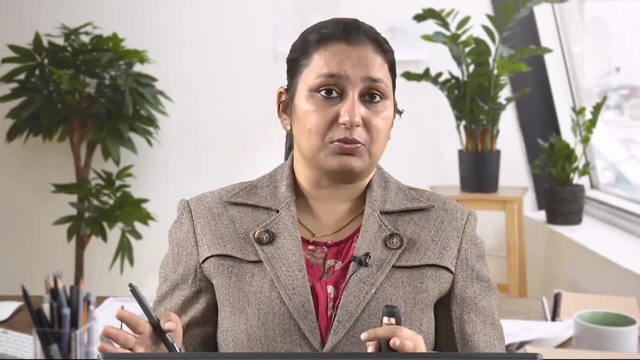 Second, the moment it is standardized it will automatically become disambiguous, but still we have to try to maintain that the drawing is not ambiguous at all. It should convey what it meant to convey and not something else. Third thing: it has to be scaled uniformly and it has the scale. 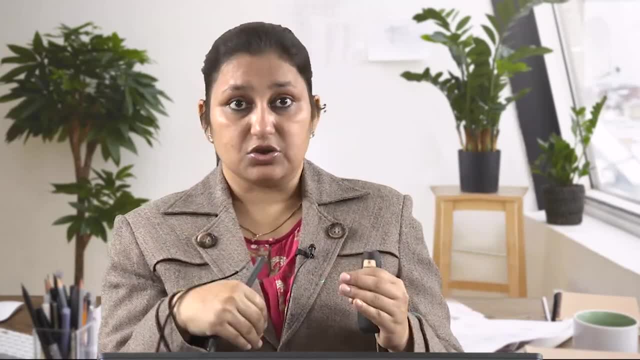 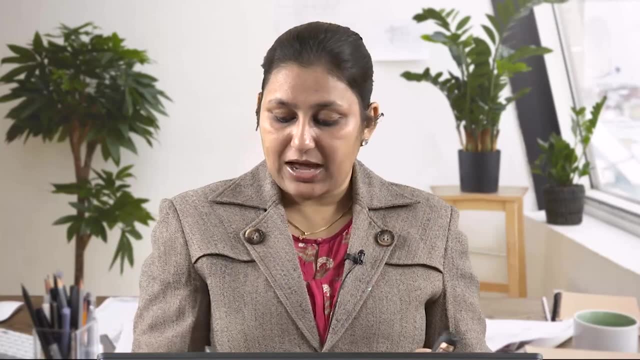 has to be clearly communicated along with the dimensions, So it has to clearly show the dimensions. Now, when I say scale, it has to be clearly communicated along with the dimensions. So when I say scale uniformly, what I mean is we could have a huge big drawing Now, if I have. 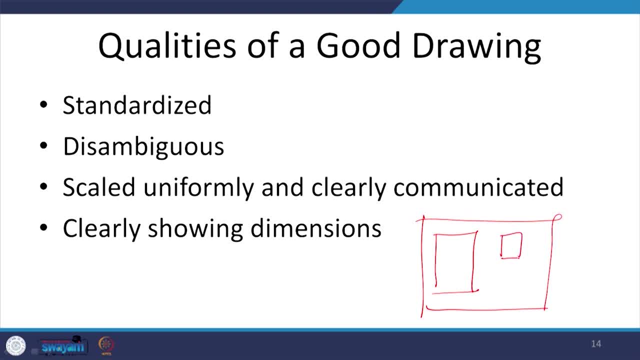 one piece of the drawing here and another piece of the drawing here. it should not have some other scale here and some other scale there. This entire thing has to have the same scale. in case it is like a blow up of this, you know a smaller part, then in that case the scale has to be. 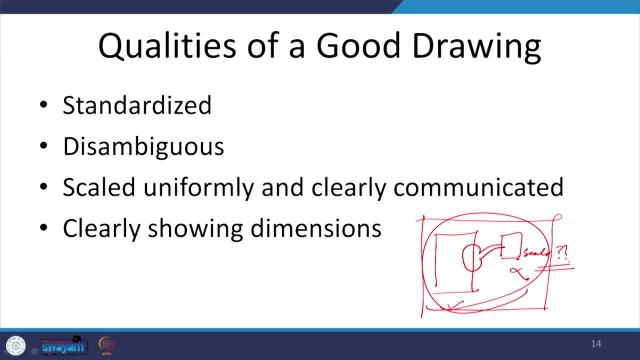 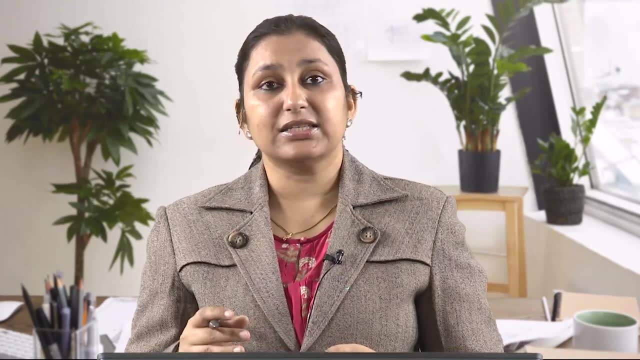 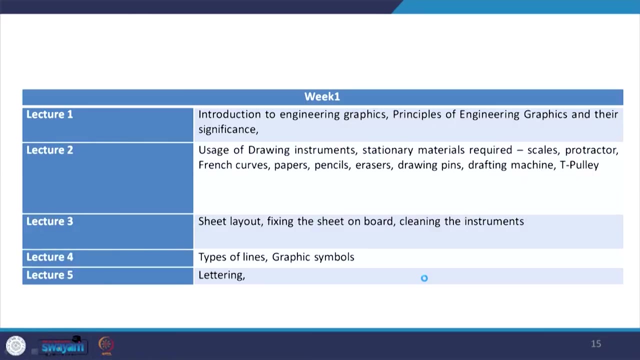 specifically mentioned. A different scale will be specifically mentioned here. Otherwise, for this entire drawing the same scale will be maintained and it will be used. So before I close this lecture here, I will quickly take you through what we are going to read in the coming weeks. So the week 1 will actually be the introduction. So 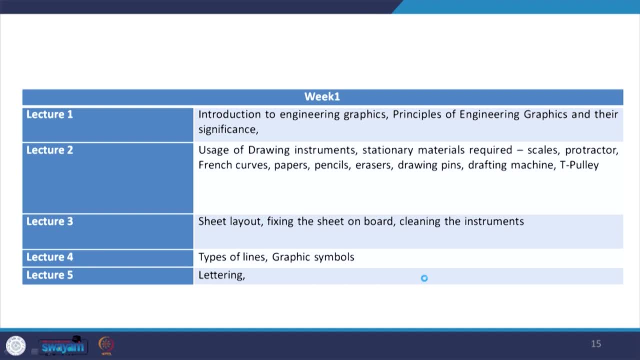 we will understand about the principles of engineering graphics, which we have covered in today's lecture. Different drawing instruments: how different stationary materials will be used, what are the purposes. different sheet layouts: how do we fix the sheet? cleaning the instruments. different types of lines and graphic symbols, lettering, 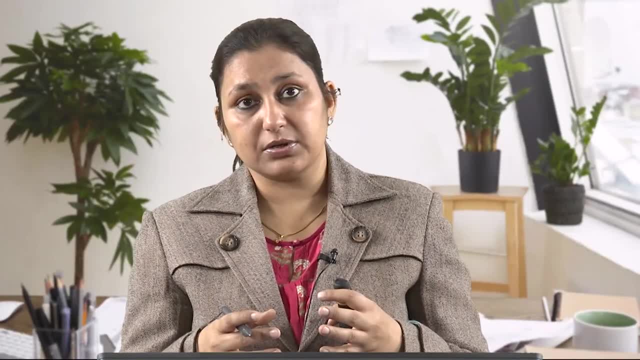 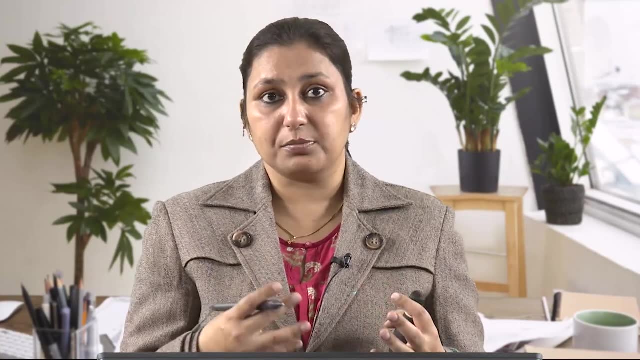 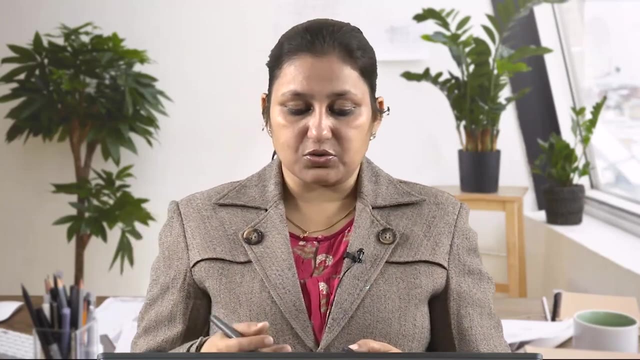 So basically the introductory stuff which you say, the vocabulary building, or I should not even vocabulary building, but in language like the understanding, knowing the alphabets and some basic words, how to put words together, something like that. In week 2, we will start with 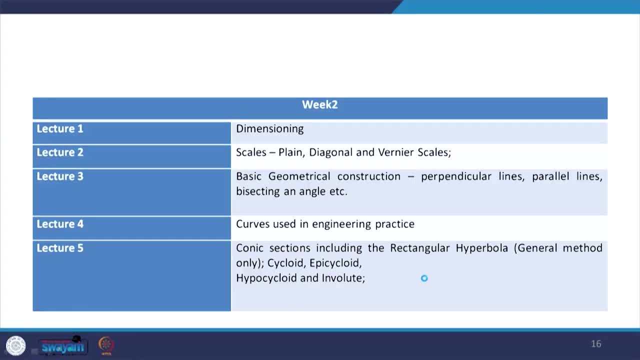 dimensioning and scales, because scales are very important. So we will understand about scales and then we will start about basic geometrical construction using these equipments And then we will go on to understand how the curves in engineering practice will be used and different conic sections. Week 3, we will start with orthographic. 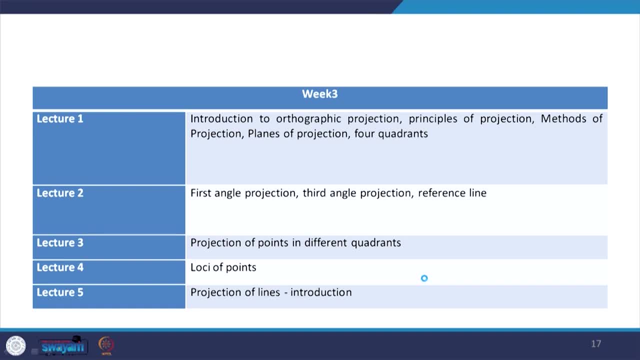 procedures. So we will start with orthographic procedures. So we will start with orthographic projections, So we will understand the orthographic projection, the principles, and then we will majorly work in first angle projection, though we will understand about first angle, third angle, both, and then we will go on to start with projection of lines. 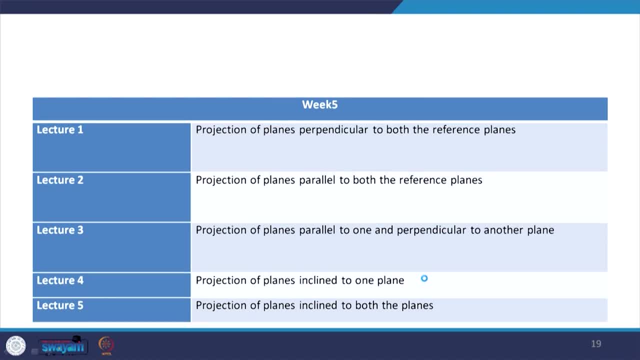 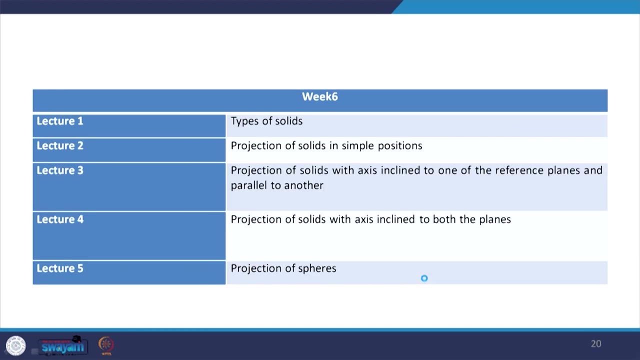 So then, week 4, we will go with projection of lines. Week 5, we will move on to projection of planes, and the complexity of these different projections will continue to increase. Week 6, we will move on to solids. From planes, we will move on to solids and the whole solids. 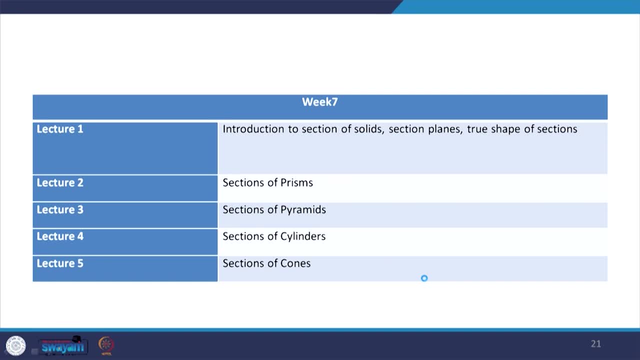 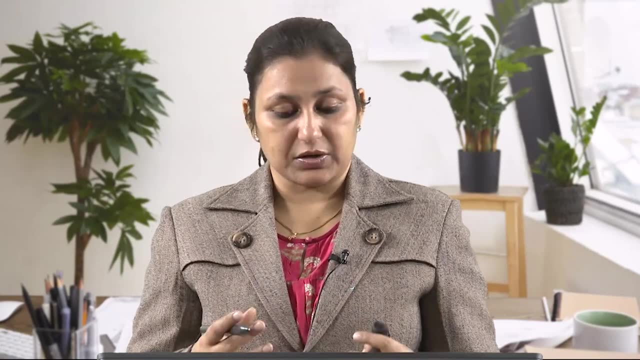 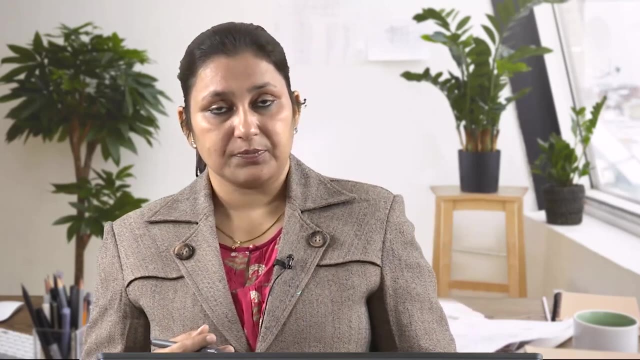 Week 7, we will look at sections of these solids. So if the solids are being cut, then what do we see? Week 8, we will move on to spherical surfaces- how do we develop different surfaces? and then intersection of these different solids. So that is all for today. I will meet you in the next. 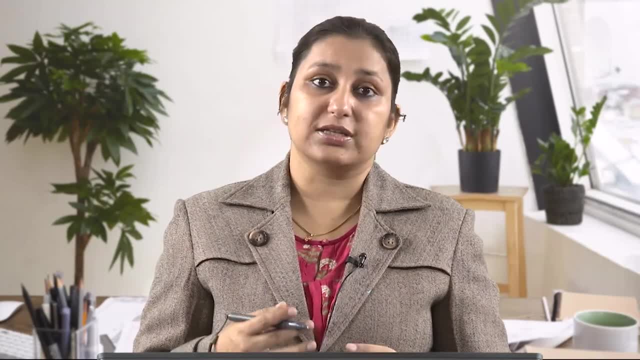 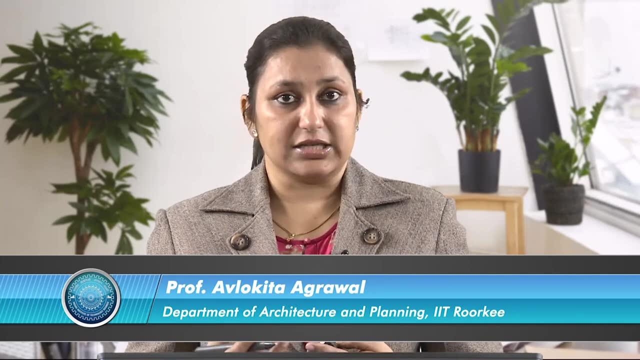 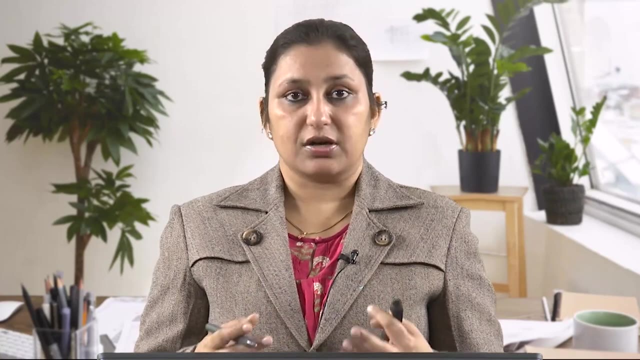 lecture where we will be seeing what are the different equipments and instruments, tools which we will be needing, stationary items to carry on with this course on engineering drawing. So, after the second lecture, I would request all of you to kindly procure these tools so that